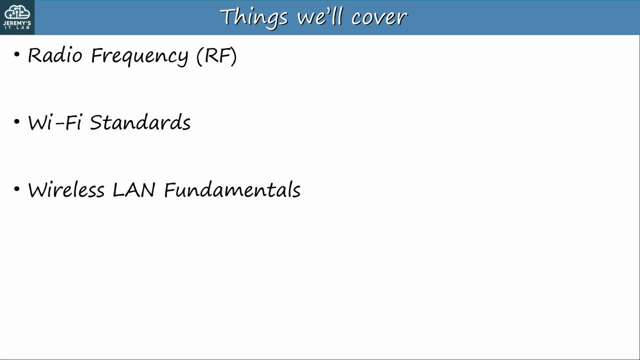 notes as you watch. When learning new concepts, taking notes is important to help you keep the new information organized without feeling overwhelmed. Make sure to watch until the end of the video for a bonus practice question from Boson Software's ExSim for CCNA. my 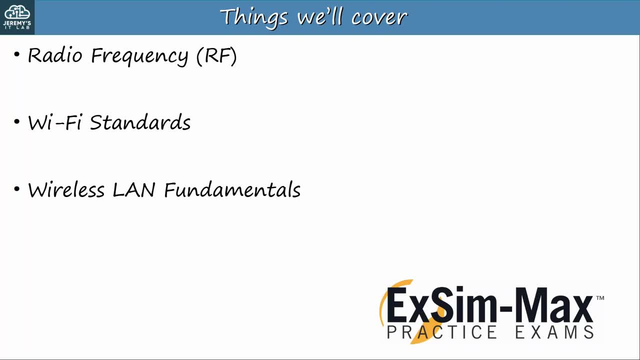 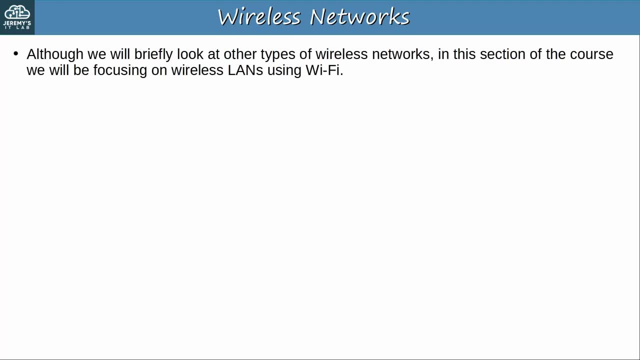 recommended practice exams for the CCNA. First, let me introduce wireless networks, specifically wireless LANs, Although we will briefly look at other types of wireless networks in this section of the course. we will be focusing on wireless LANs using Wi-Fi, because that's what you need to know for the CCNA. 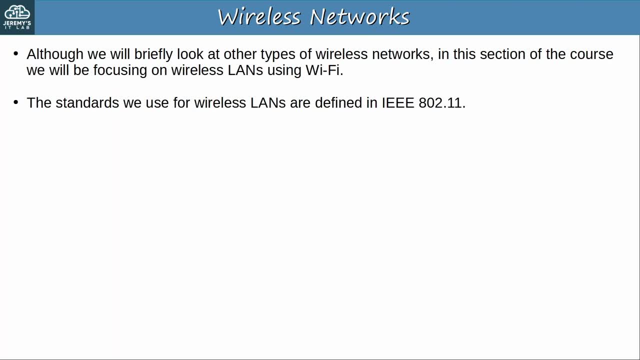 The standards we use for wireless LANs are defined in IEEE 802.11, just like how wired Ethernet LANs are defined in IEEE 802.3.. Note that the term Wi-Fi is a trademark of the Wi-Fi Alliance, which is not directly connected to the IEEE. The Wi-Fi Alliance. 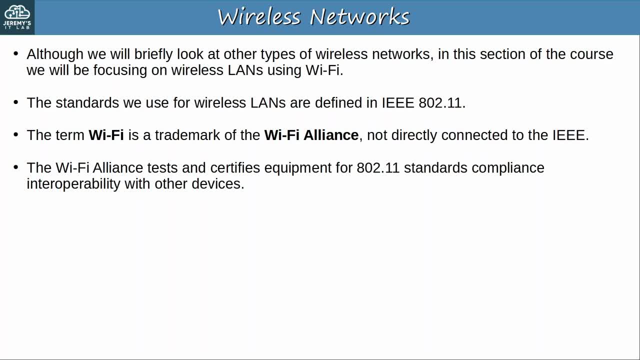 tests and certifies equipment for 802.11 standards compliance and interoperability with other devices. Devices which have been Wi-Fi certified can use the Wi-Fi certified mark like this, For example: this is a photo of the backside of one of the Cisco wireless access points that I. 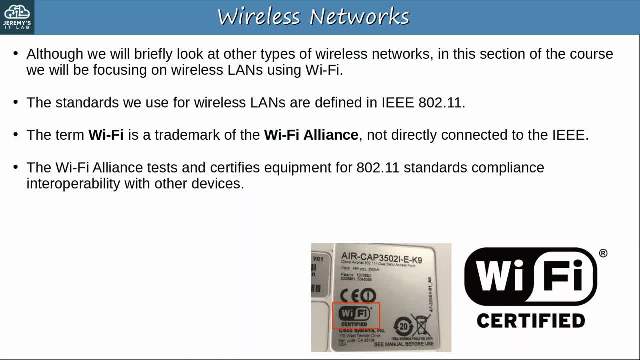 will be using to make these videos. As you can see, it has been certified by the Wi-Fi Alliance. So, although the Wi-Fi Alliance certifies devices for compliance with the 802.11 standards, Wi-Fi isn't technically the correct term to refer to 802.11 wireless LANs. 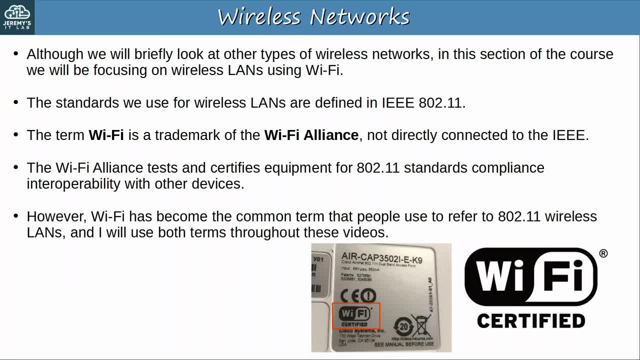 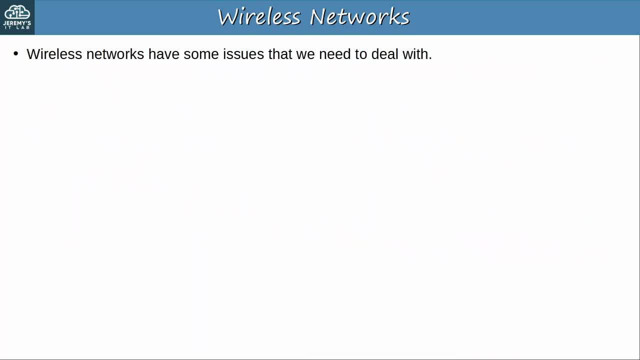 However, Wi-Fi has become the common term that people use to refer to 802.11 wireless LANs, and I will use both terms throughout these videos. Wireless networks have some issues that we need to deal with. First of all, all devices within. 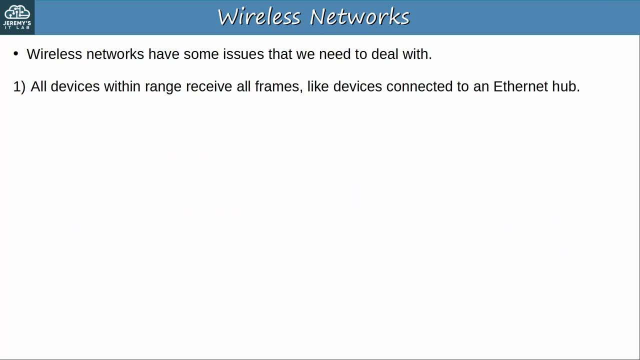 range receive all frames like devices connected to an Ethernet hub. When using an Ethernet switch, the switch is able to forward from the Ethernet hub to the Ethernet hub. In addition, switches allow devices to function using full-duplex, so devices can both send and. 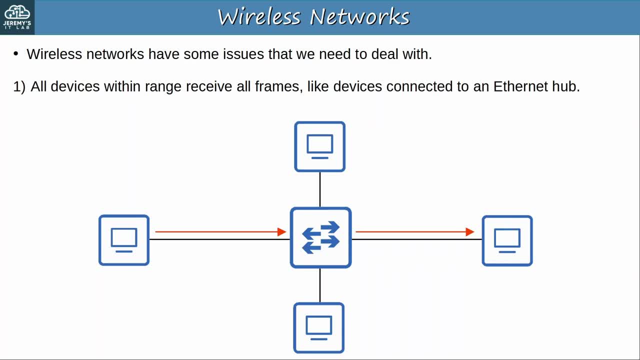 receive frames at the same time and collisions shouldn't occur unless there is some problem in the network. However, when using an Ethernet hub, the hub will always flood all frames it receives and collisions can occur when multiple devices try to send and receive traffic at the same time. 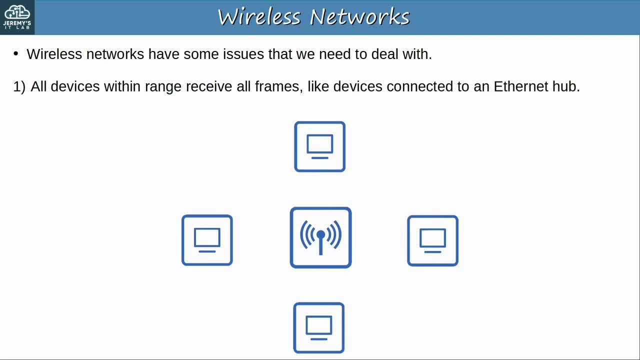 Like devices connected to an Ethernet hub. when a wireless device transmits a frame, all wireless-enabled devices within range will be able to pick up that frame. The signal isn't contained within a physical wire, because the signal consists of electromagnetic waves radiating out from the transmitting device. 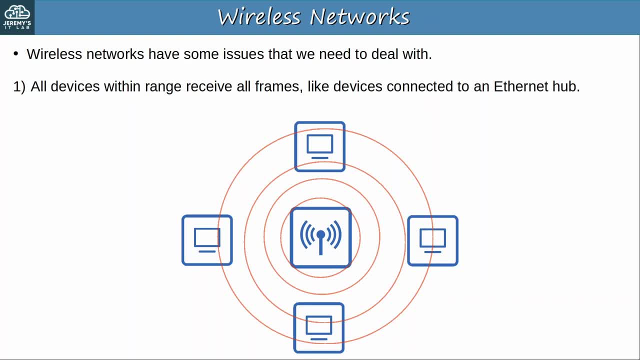 This can lead to data privacy concerns, as well as collisions, when devices communicate on the same channel at the same time. So, because all devices within range receive the frames, privacy of data will be limited to the same channel at the same time. So a network tailoring data within the LAN is a greater concern In wired networks. 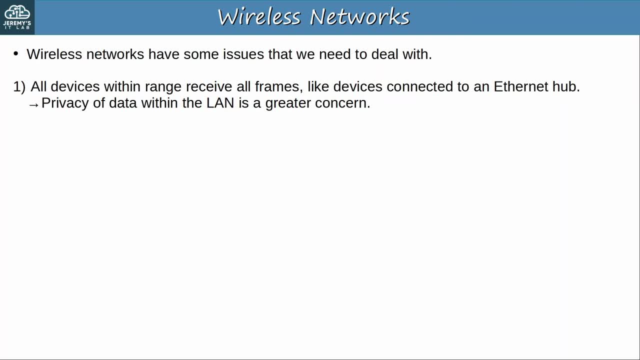 we don't usually encrypt data within the LAN, only when sending data over a shared network such as the Internet. However, for wireless networks, it is very important to encrypt data even within the LAN, or else anyone with a device in range of the transmitter can access that data. 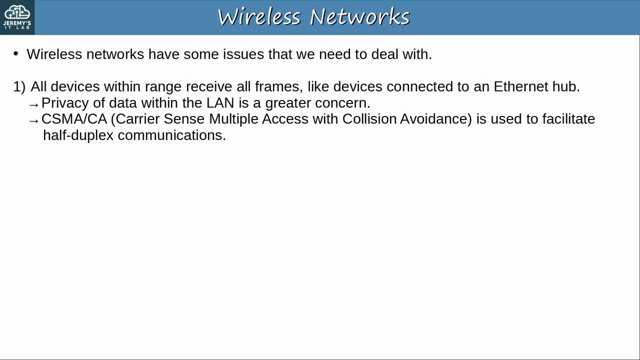 Also to avoid collisions and facilitate half-duplex communications. CSVMA-CA carrier sense. multiple access with collision avoidance is even more important if these networks are smart enough to snake online traffic reasons, even most Rashtrons are unable to make online cake. 有她s' comm십资 Oberteäm. 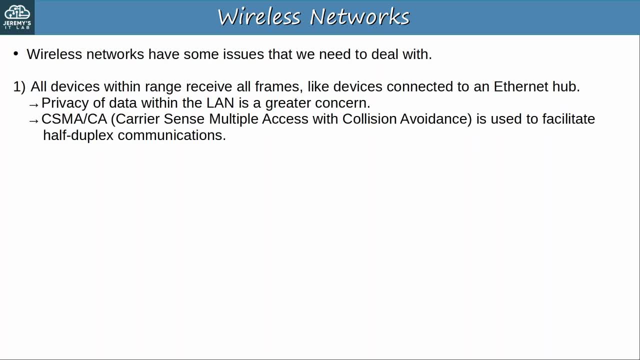 is used. That's similar to another term I mentioned earlier in the course. CSMA-CD is used in wired networks to detect and recover from collisions. CSMA-CA is used in wireless networks to avoid collisions before they occur. Basically, when using CSMA-CA, a device will 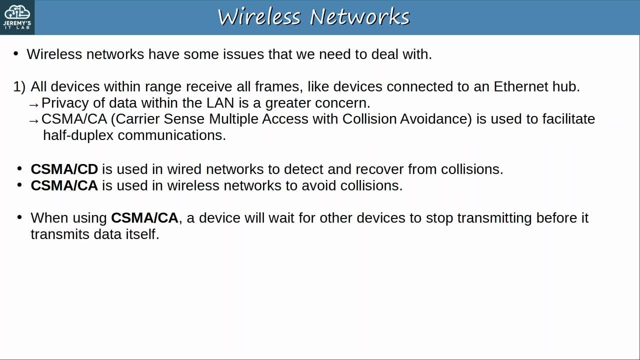 wait for other devices to stop transmitting before it transmits data itself. Let's look at a simple flowchart of the process. The transmitting device assembles the frame, prepares it to be sent, Then it listens to check if the channel is free. If the channel is not, 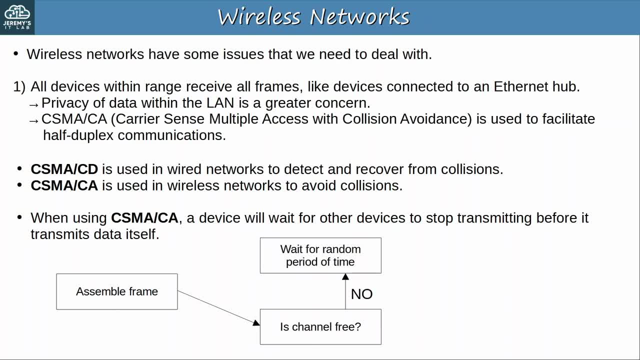 free, it will wait for a random period of time, Then it will listen again. If the channel is free this time, it will transmit the frame. Note that this is a simplification of the process and there is an optional feature in which the transmitting device sends a request-to-send. 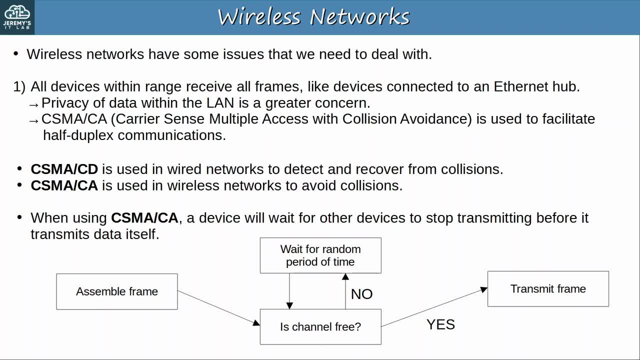 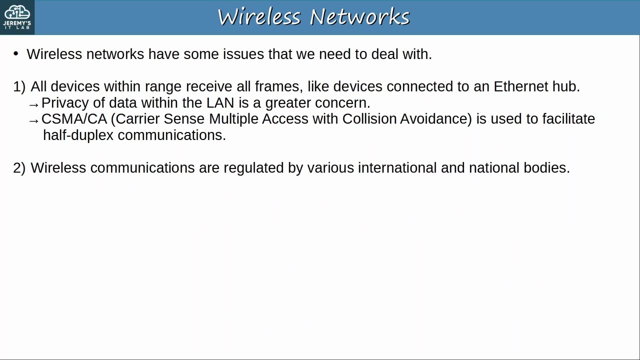 RTS packet to the channel. But this is just extra information, not something you need to know for the CCNA, But make sure you know the term CSMA-CA and that it is used in wireless LANs to avoid collisions. Another issue that we must deal with is that wireless communications are regulated by various 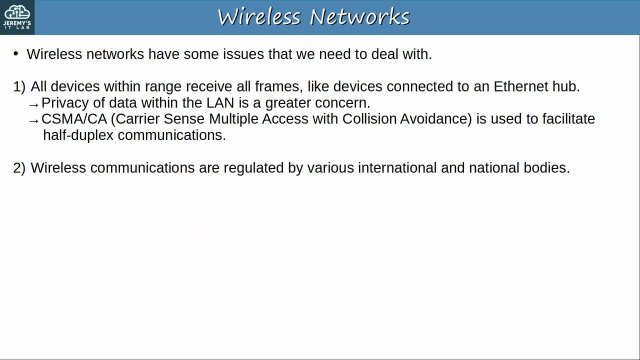 international and national bodies. You aren't allowed to transmit data on any channel you want, And which channels you are allowed to use can vary depending on the country. Fortunately, the 802.11 standard outlines which frequencies can be used for wireless LANs and devices. 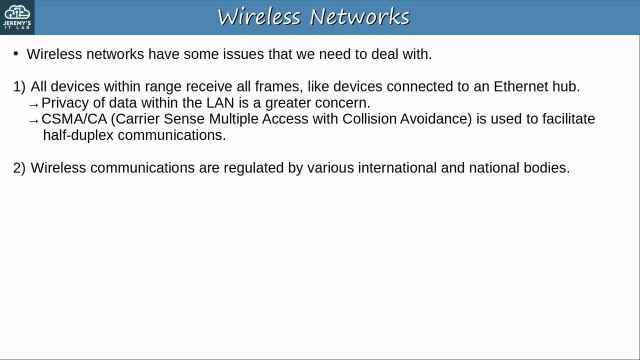 are designed to use those frequencies. We also must consider the wireless signal coverage area. In wired connections we do have to consider the cable length and in some cases electromagnetic interference. But with wireless connections there are other factors. we must consider, First of all, the signal range, how far the signal can actually travel- And there are. 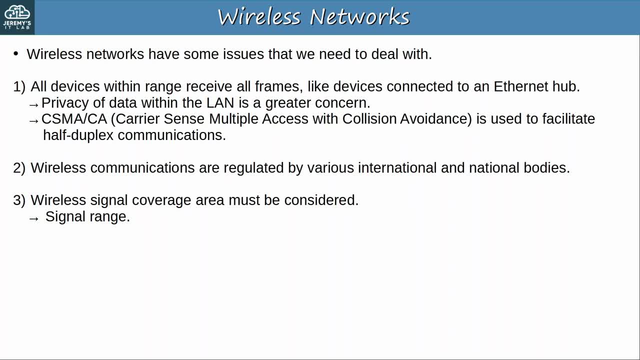 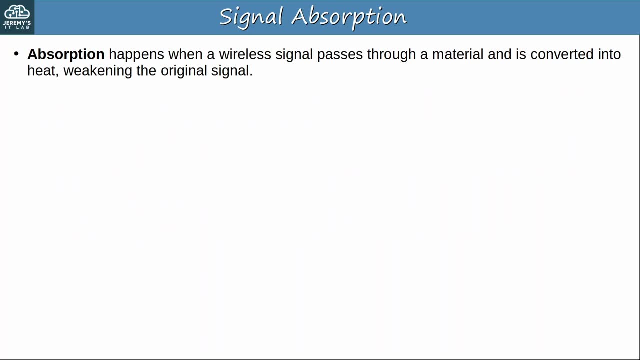 several factors that affect how far a signal can travel intact: Absorption, reflection, refraction, diffraction and scattering. Let's briefly look at each of them. Absorption happens when a wireless signal passes through a material and is converted into heat, weakening the original signal. Here's an example. By the way, I took this screen. 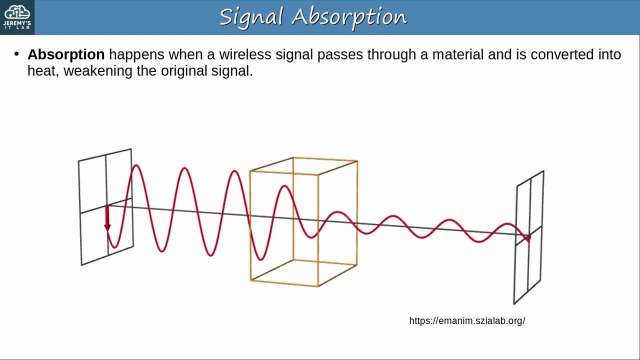 shot from MNM, which can be used to animate electromagnetic waves. Check out the link I put below the image. to use MNM it's free. So a wireless access point sends a signal, but the receiving laptop is on the other side of a wall. The wall absorbs some of the signal. 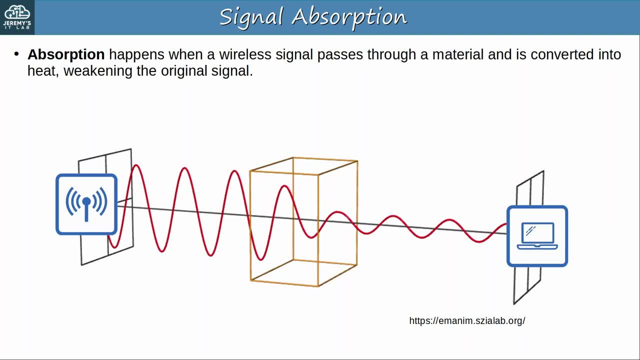 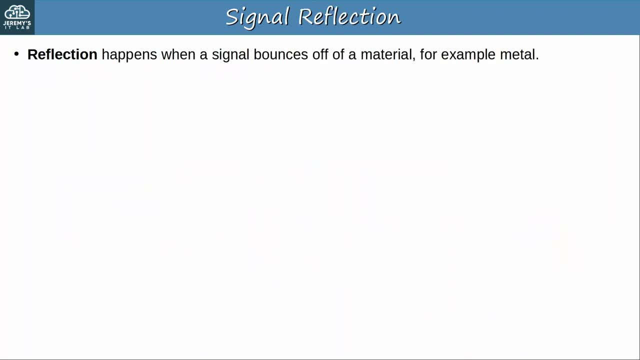 resulting in a weaker signal by the time it reaches the laptop. That's absorption. Reflection happens when a signal bounces off of a material, for example metal. This is why Wi-Fi reception is usually poor in elevators, because the signal bounces off the metal and 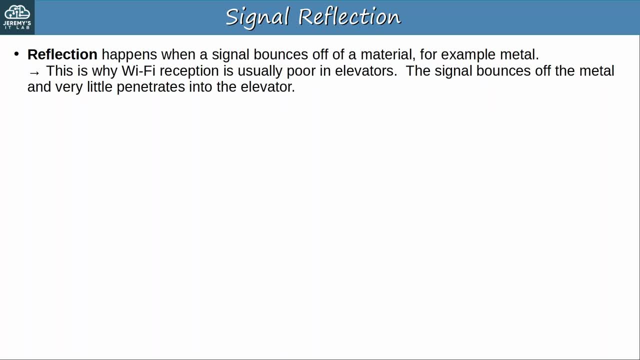 very little penetrates into the elevator. For example, if there is a metal wall between an AP and a laptop, most likely the laptop will not receive a good signal from the AP because much of the signal will bounce off of the wall. Refraction happens when a wave. 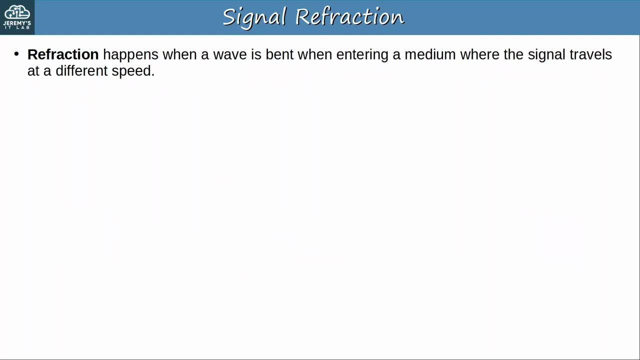 is bent when entering a medium where the signal travels at a different speed. For example, glass and water can refract waves. Try putting a straw into a clear glass of water. It will appear as if the straw is bent. That's because the light waves travel at a different speed in water than in air. That's 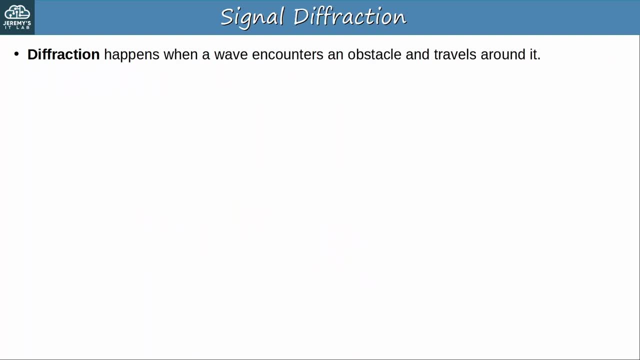 refraction. Diffraction happens when a wave encounters an obstacle and travels around it. This can result in blind spots behind the obstacle. For example, this PC is blocked by some object and the signals from the wireless access point travel around the object to some degree. This 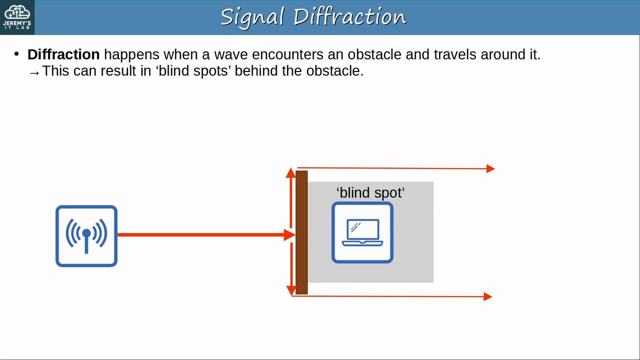 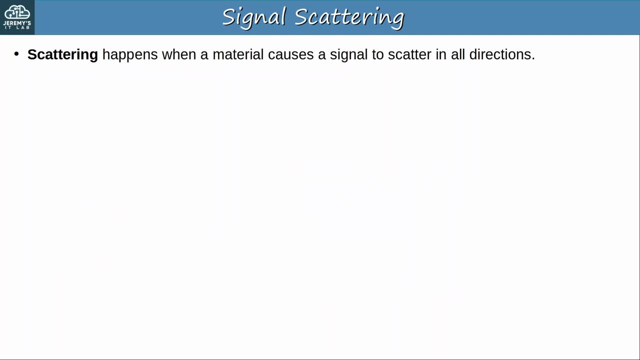 is diffraction, but the PC is in a blind spot and doesn't receive sufficient signal from the access point. That's diffraction. Scattering happens when a material causes a signal to scatter in all directions. Dust, smog, uneven surfaces etc can cause scattering. 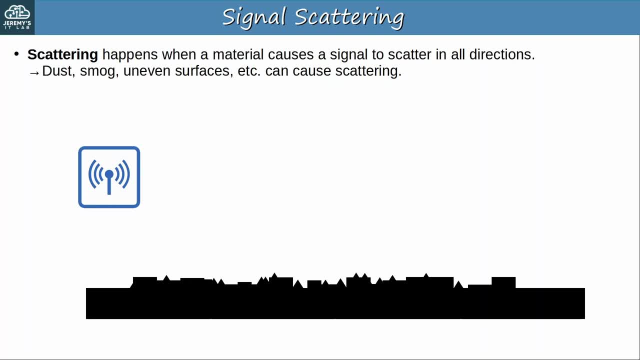 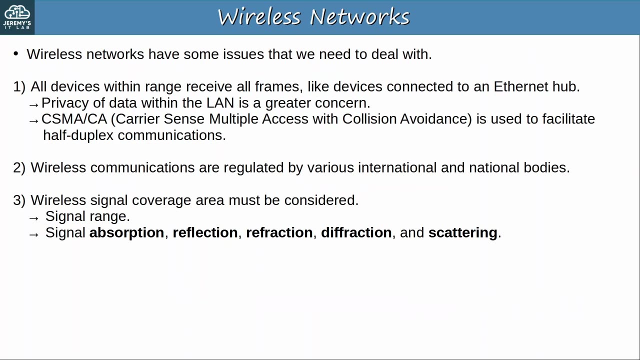 Forgive the unprofessional diagram again, but when a signal from this wireless access point strikes this uneven surface, the signal is scattered in all directions. That's scattering All of those Absorption, reflection, refraction, diffraction and scattering can affect the quality of. 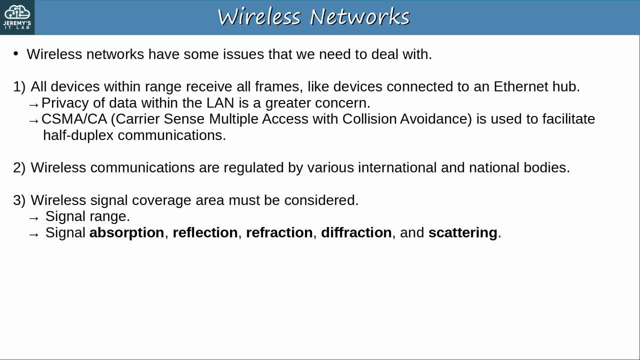 a wireless signal. When planning the positioning of wireless access points for a network, you have to take all of these into account. One more issue I want to mention is interference. Other devices using the same channels can cause interference, For example, a wireless LAN in your neighbor's house or apartment. 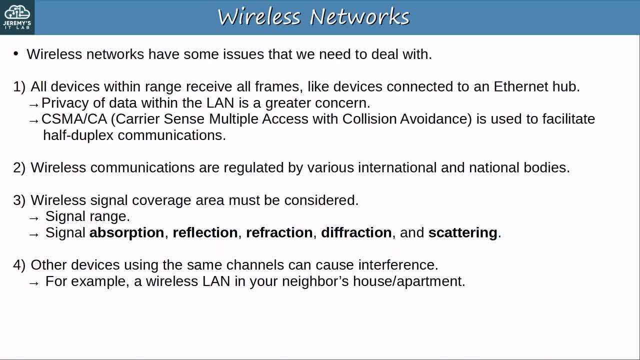 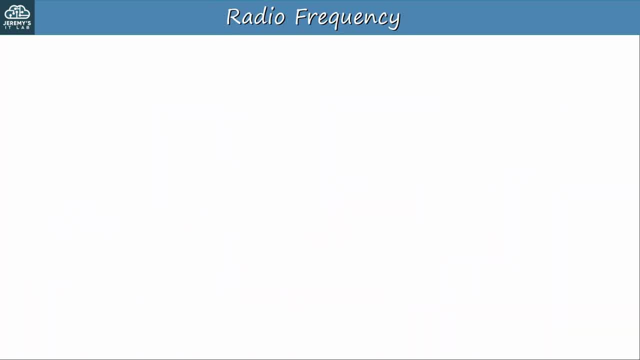 So I think you can see that there are various things we have to take into concern, but I think this is a very important issue when building a wireless network that we don't have to think about with wired networks. Now let's talk about radiofrequency and electromagnetic waves in general To send wireless signals. 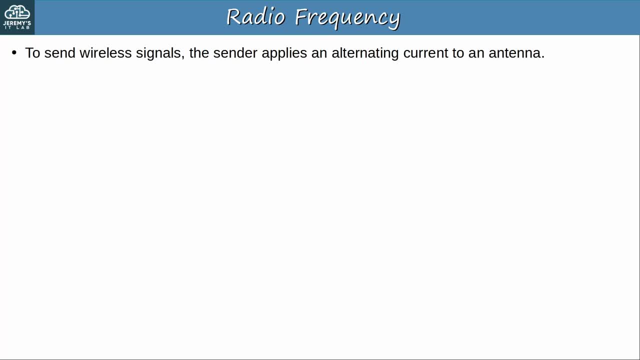 the sender applies an alternating current to an antenna, This creates electromagnetic fields which propagate out as waves. Electromagnetic waves can be measured in multiple ways, for example amplitude and frequency. Amplitude is the maximum strength of the electric wave. This is the maximum strength of the electrical wave. Amplitude is the maximum strength of. 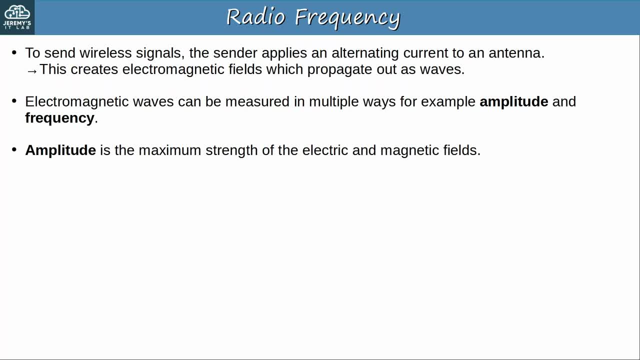 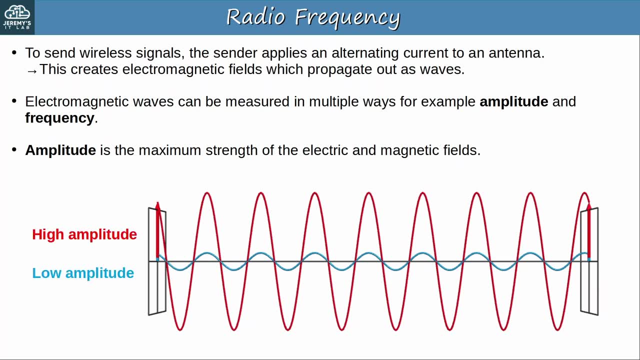 the electric wave. This is the maximum strength of the electromagnetic wave. Amplitude is the maximum strength of the electric and magnetic fields. For example, look at these two waves: The red one has a higher amplitude and the blue one has a lower amplitude, Although these 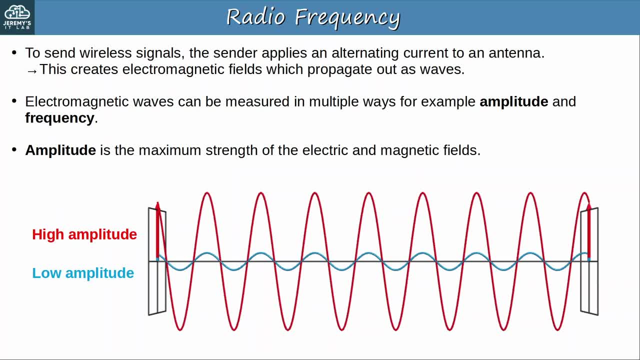 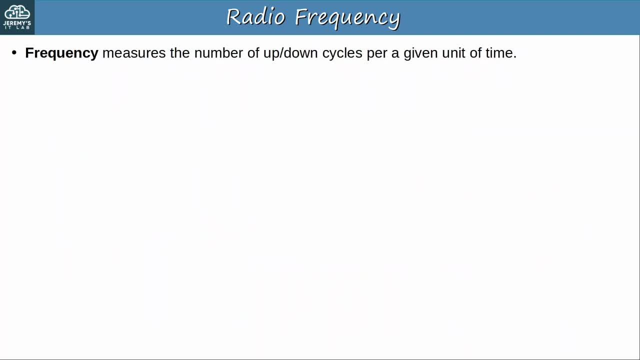 two waves have different amplitudes. they have the same frequency, which is the next term. we'll look at Frequency measures, the number of up-down cycles per a given unit of time. The most common measurement of frequency is Hertz. Hertz is simply the number of cycles. 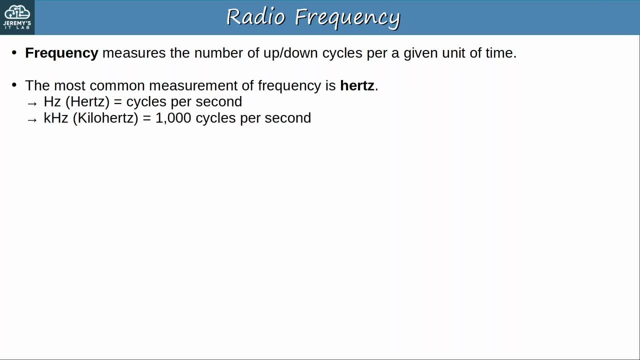 per second. Then of course there are kilohertz, thousands of cycles per second. megahertz, millions of cycles per second. gigahertz, billions of cycles per second. and terahertz, trillions of cycles per second. Of course there are. 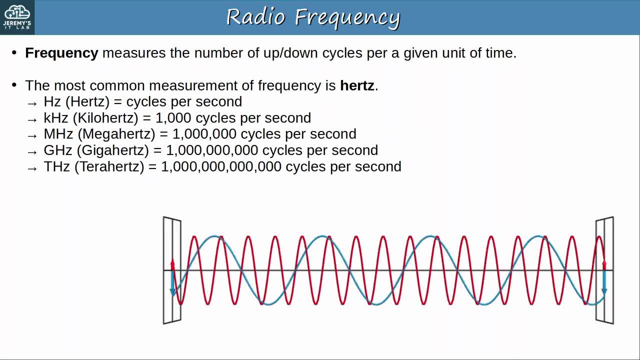 more, but these are the common ones. Look at these two waves. Although they both have the same amplitude, this time the red one has a higher frequency and the blue one has a lower frequency. The red one goes through more cycles per second than the blue one. 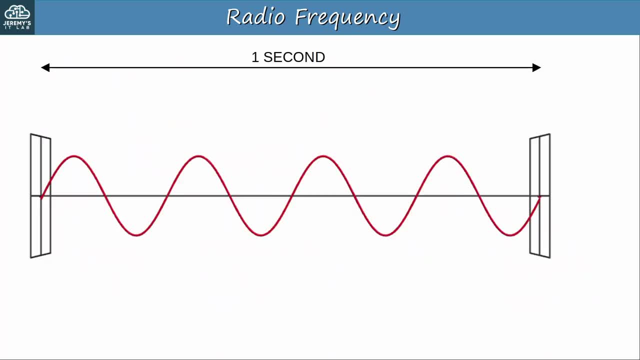 Look at this wave. Let's say this represents the frequency of the electric wave. This is 1 second. Let's say this represents 1 second. What is the frequency of this wave? Well, this is one cycle, this is a second cycle, a third cycle and a fourth cycle. So this 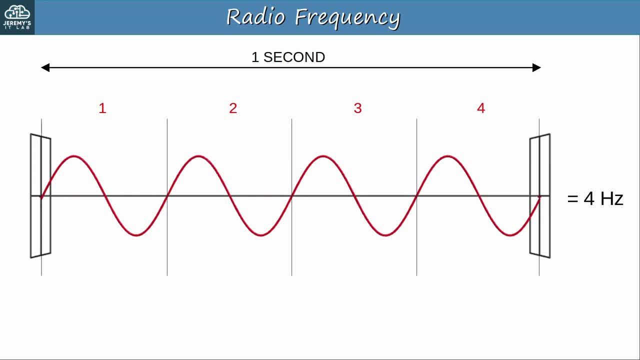 is 4 cycles per second, 4 Hertz. By the way, another important term is period: the amount of time of one cycle. So if the frequency is 4 Hertz, the period is 0.25 seconds one. 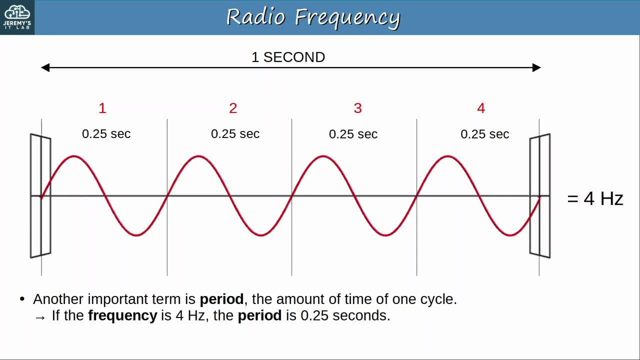 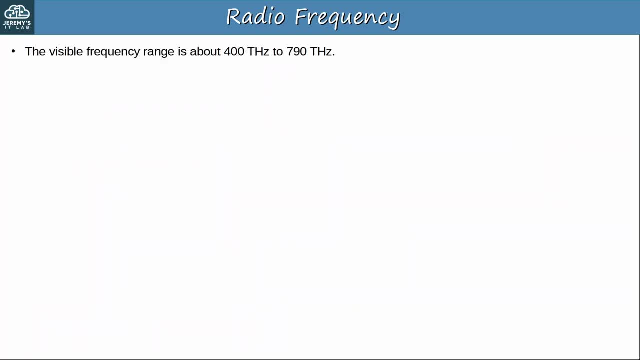 quarter of one second, because 4 cycles occur in one second. The visible frequency range is from about 400 terahertz to 790 terahertz, but the range we are concerned with radio frequency is from about 30 Hertz to 300 gigahertz, and 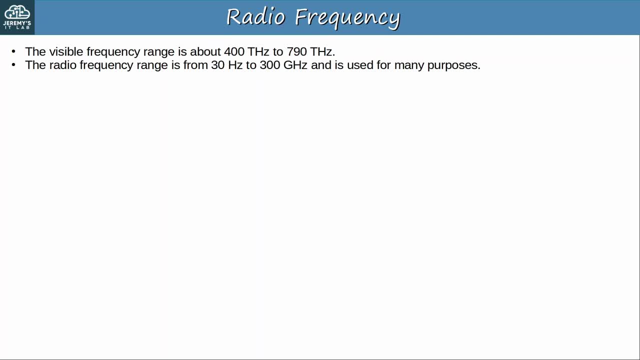 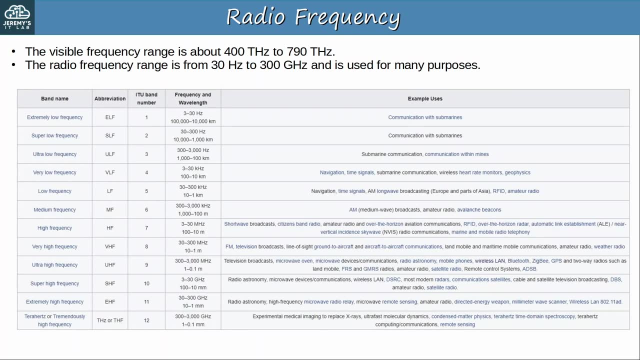 it's used for many purposes. Actually, we're only concerned with a couple small bands of this range, Thanks to Wikipedia for this chart of the radio frequency spectrum. The text is a bit small so it might be hard to read, but that's okay. I just want to point out. 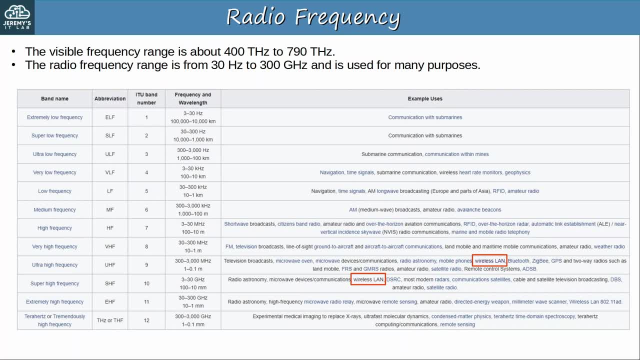 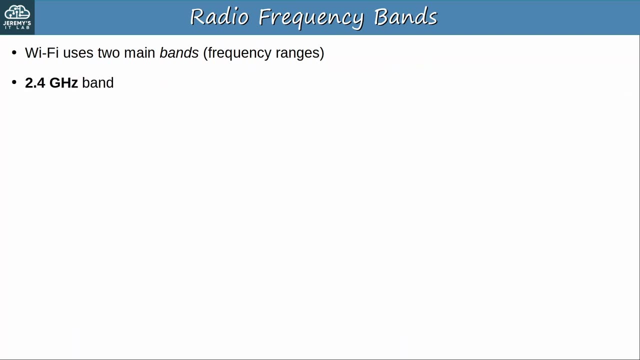 that the frequency range is used for wireless LANs. IEEE 802.11 Wireless LANs use a few sections of the ultra-high frequency and super-high frequency ranges. Wi-Fi uses two main bands, meaning frequency ranges. First is called the 2.4 GHz band. 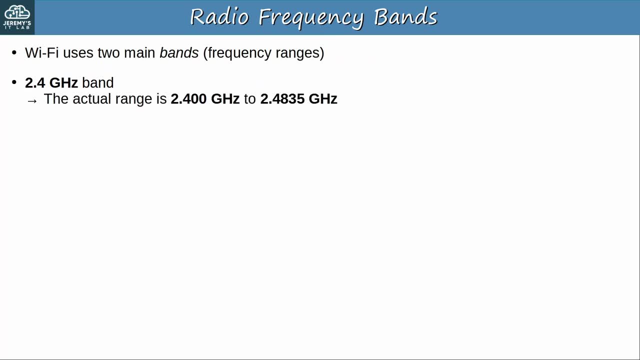 The name is 2.4 GHz, but the actual range is from 2.4 GHz to 2.4835 GHz. Then there is the 5 GHz band. This time it's 2.4 GHz, The actual range is from 5.150 GHz to 5.825 GHz, but it's further divided into four smaller 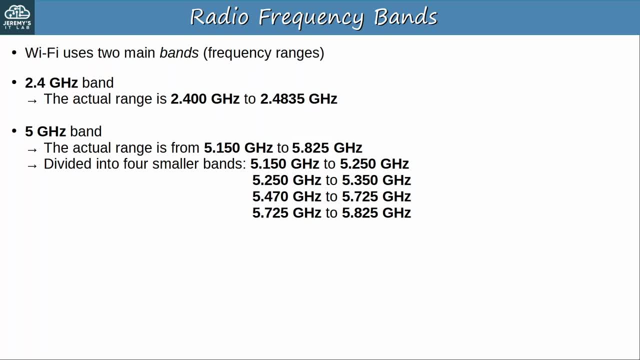 bands. Note that you don't have to memorize any of these band ranges, just remember the two main ones: 2.4 GHz and 5 GHz. If you want to become a wireless network expert, you might want to remember the exact ranges and bands, but for the CCNA that's not necessary. The 2.4 GHz band typically provides a range of about 50 GHz, but it's not necessary to memorize the exact ranges and bands. The 2.4 GHz band typically provides a range of about 50 GHz, but it's not necessary to memorize any of these bands. The 2.4 GHz band typically. 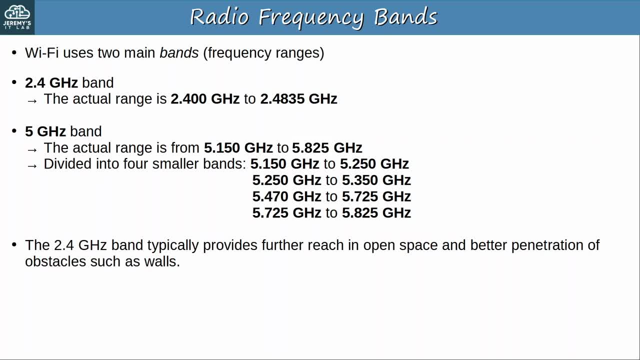 provides further reach in open space and better penetration of obstacles such as walls. However, more devices tend to use the 2.4 GHz band, so interference can be a bigger problem compared to the 5 GHz band. Modern devices typically support both, and it's up to you which you 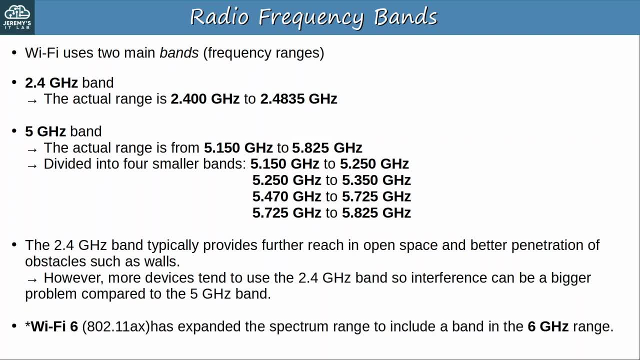 want to use. Note that Wi-Fi 6,, which is IEEE standard 802.11ax, has expanded the spectrum range to include a band in the 6 GHz range. I'm not sure if you'll be asked about the 6 GHz range in the CCNA exam, but I'm. 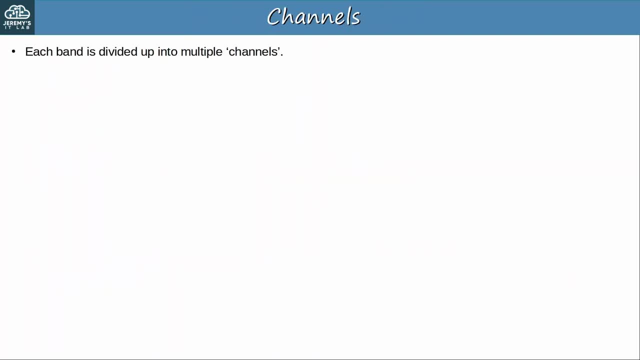 mentioning it just in case. Now each band is divided up into multiple channels and devices are configured to transmit and receive traffic on one or more of these channels. I say or more, because something called channel bonding can be used to combine channels together. but I don't think you. 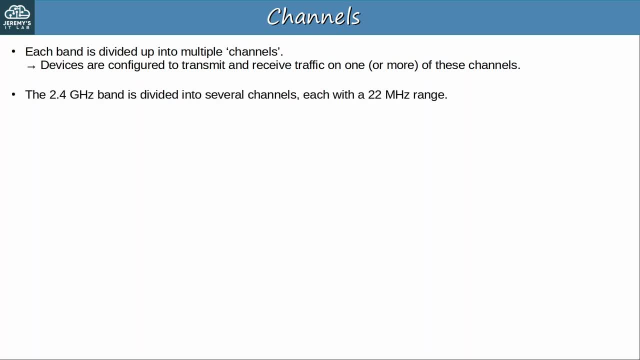 need to know that for the CCNA, For example, the 2.4 GHz band is divided into several channels, each with a 22 MHz range. Here are the channels, and note that it differs by country, Thanks to Wikipedia for the chart again, by the way, 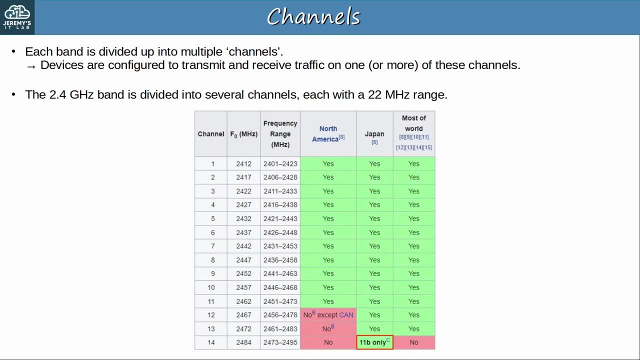 Note that the 11B- only here for channel 14 in Japan- refers to 802.11b, which is an old and slow standard not used much anymore Now. an important aspect of these channels is that they overlap, For example, channel. 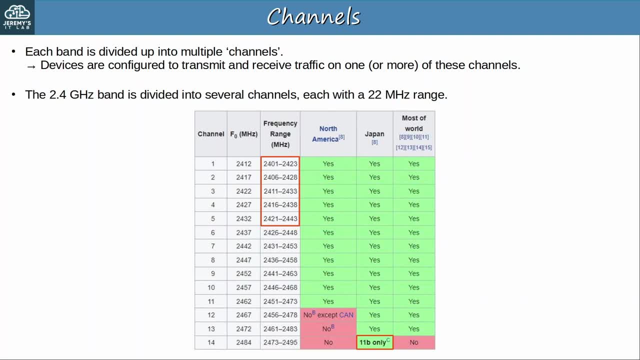 1 is from 2401 MHz to 2420 MHz, 23 MHz, which has some overlap with channels 2,, 3,, 4, and 5.. To avoid interference between adjacent wireless access points, we have to carefully choose. 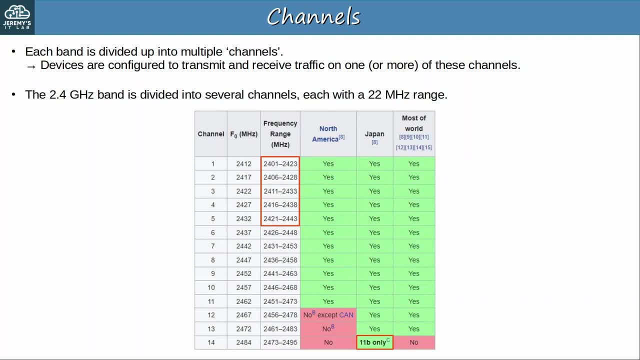 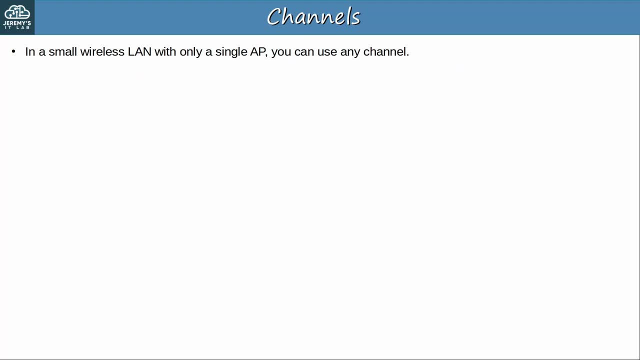 which channels we configure our access points to use. In a small wireless LAN with only a single access point, you can use any channel because there are no other access points that can cause interference. However, in larger wireless LANs with multiple APs, it's important that adjacent APs don't. 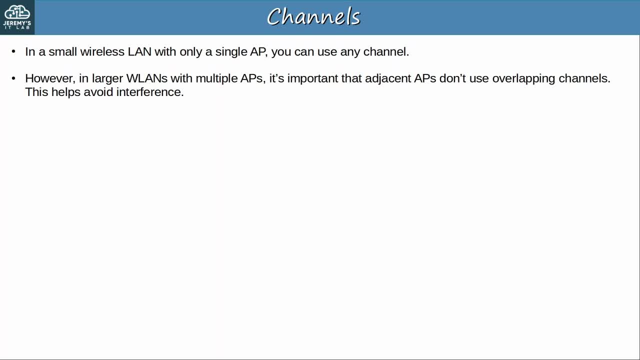 use overlapping channels. This helps avoid interference between devices transmitting on the same channel. If overlapping channels are used, it will result in reduced performance and a worse user experience. In the 2.4 GHz band, it is recommended to use three channels: 1, 6, and 11.. 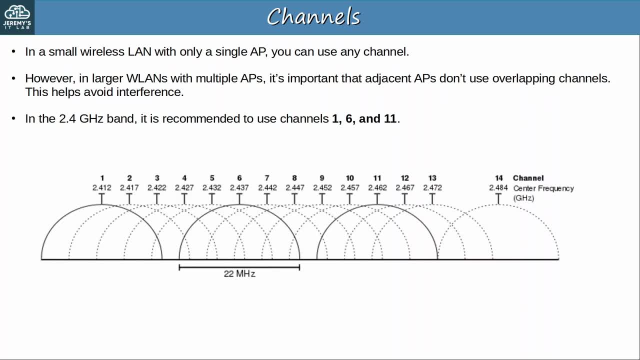 Here is a diagram of the channels in the 2.4 GHz band. Notice that channels 1,, 6, and 11 don't overlap with each other, So we can have an AP with only a single access point, An AP using channel 1,, an AP using channel 6, and an AP using channel 11, and they won't. 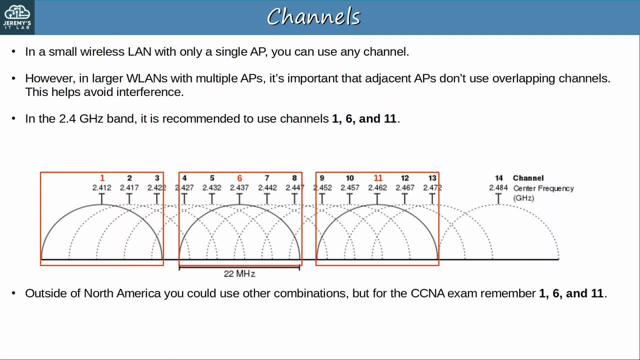 interfere with each other. Note that outside of North America you can use other combinations, but for the CCNA you should really remember the 1,, 6, and 11 combination. And as for the 5 GHz band, it consists of non-overlapping channels, so it is much easier. 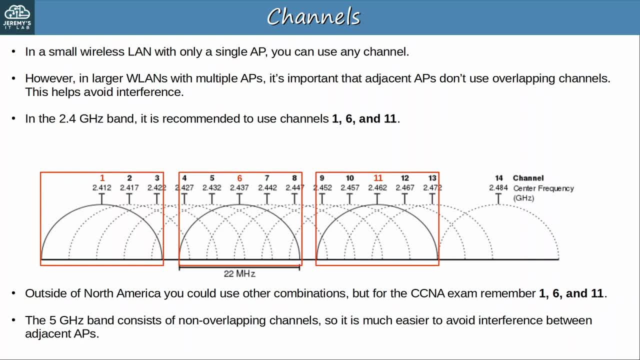 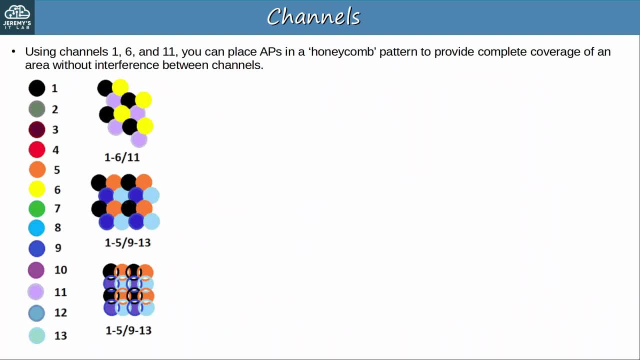 to avoid interference between adjacent wireless access points. So that's it. Thanks for watching. If you want to see channels in the 2.4 GHz band, you can place APs in a honeycomb pattern to provide complete coverage of an area without interference between channels. 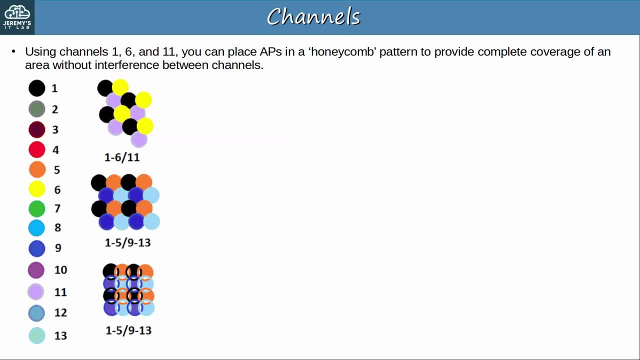 The diagram on the left shows how you can do that with channels 1,, 6, and 11, as well as other patterns for those outside of North America. Here's a large version of the 1,, 6,, 11 honeycomb pattern. 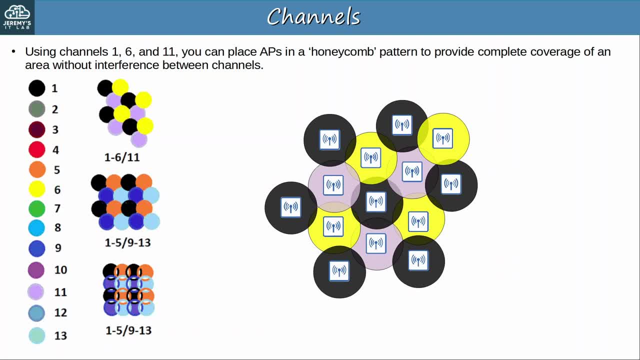 Note that the coverage area of each AP overlaps to provide complete coverage of the area, but the frequencies don't overlap, which helps to avoid interference between channels. When you have to provide wireless coverage over a large space, you should arrange your access points like this: 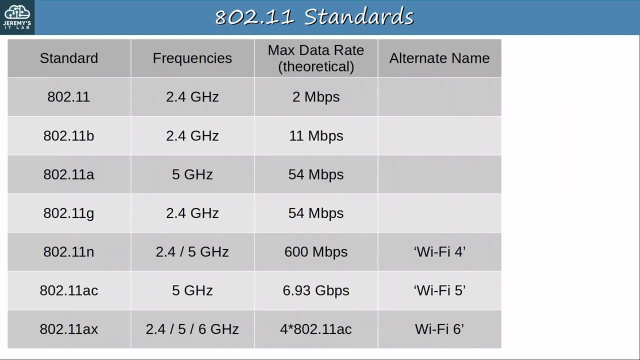 Just like there have been various 802.3 Ethernet standards, there are plenty of 802.11 Wi-Fi standards too that use different frequencies and provide different data rates, Starting with the original 802.11, which was released in 1997, all the way to 802.11aX. 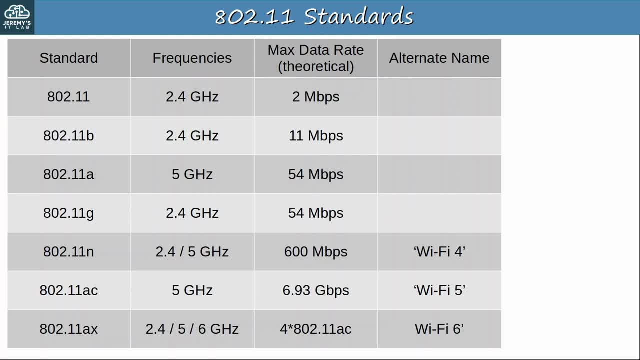 also known as Wi-Fi 6, which was released in 2019,. here are the 802.11 standards you should know. I know it's a lot of work, but I do recommend memorizing these standard names, the frequencies they use and their maximum theoretical data rates for the test. 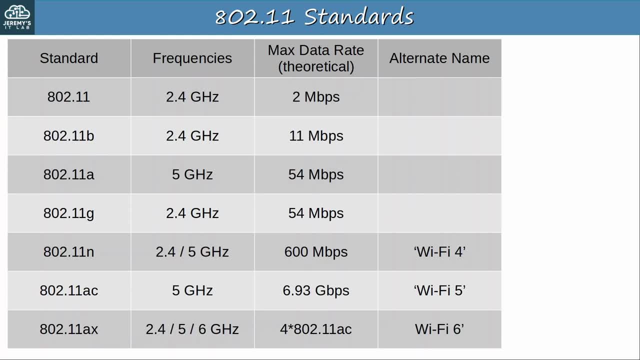 Note that these maximum data rates are theoretical For many reasons. you're probably going to get much lower data rates than the theoretical maximums. Also, notice that 802.11aX is not the maximum data rate. It's the maximum theoretical data rate. Note that 802.11aX is not the maximum theoretical data rate. Note that 802.11aX is not the maximum theoretical data rate. Note that 802.11aX is not the maximum theoretical data rate: See 802.11aX is not the maximum theoretical data rate. 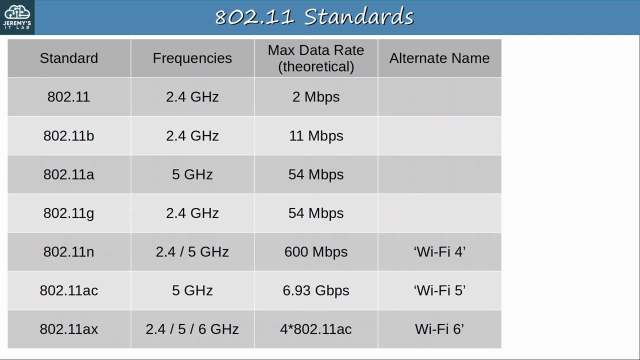 So we're using 802.11 as the textbook gia. It's still below the levels of a universality. so howPSH can beけれallyaratable and controlled like this, But the wife can still do more Right. 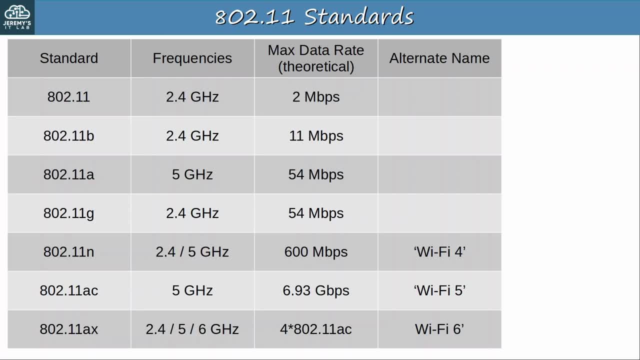 So here's the chalkboard that's been created to illustrate statka Test umine. Let's just use the number for TestMap as the standard and then we have the answer for testMap. Nina, the quizzes Beautiful. So I recommend checking which standards are supported before you buy a device. 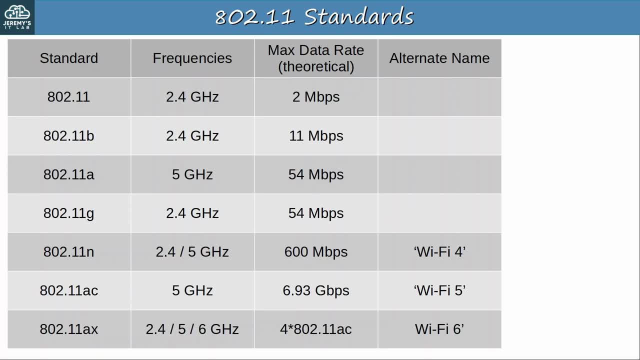 Also for some homework. try looking up the Wi-Fi standards supported by the wireless devices you own. For example, if you have an iPhone, you can check Apple's website to see which standards it supports. Here's an example for the iPhone X. 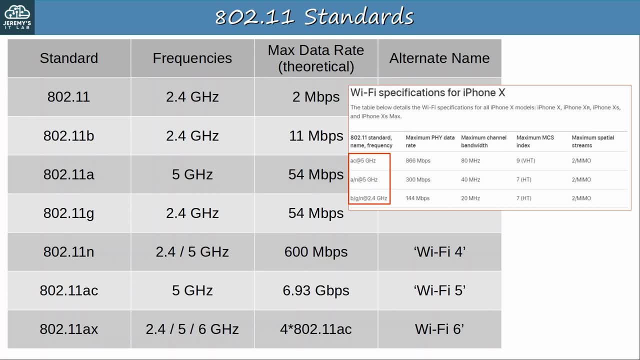 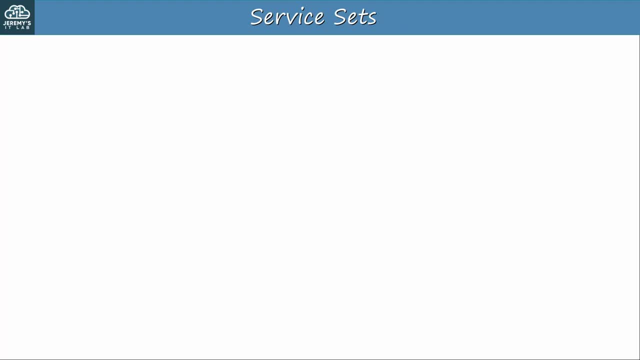 It supports 802.11a b, g, n and ac. Finally, let's look at another important part of 802.11, service sets. 802.11 defines different kinds of service sets, which are groups of wireless network. 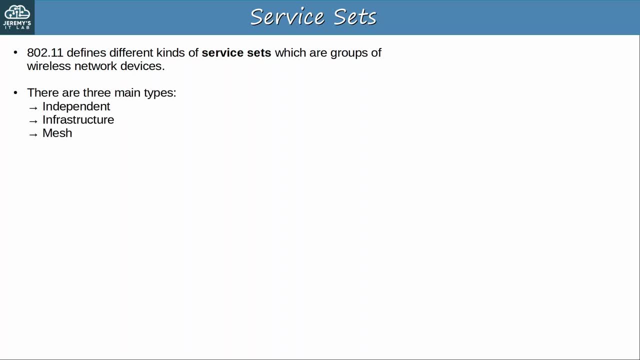 devices. There are three main types: independent service sets, infrastructure service sets and mesh service sets. All devices in a service set share the same SSID- service set ID- You might have heard that term before. The SSID is a human service. 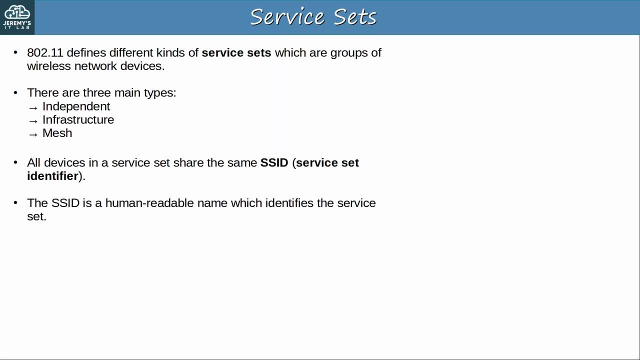 It's a human-readable name which identifies the service set, And it does not have to be unique, although it's best to configure unique SSIDs, since that's what you'll be looking at when you select which network to connect to. Here are the SSIDs my phone can detect as I sit here at my desk. 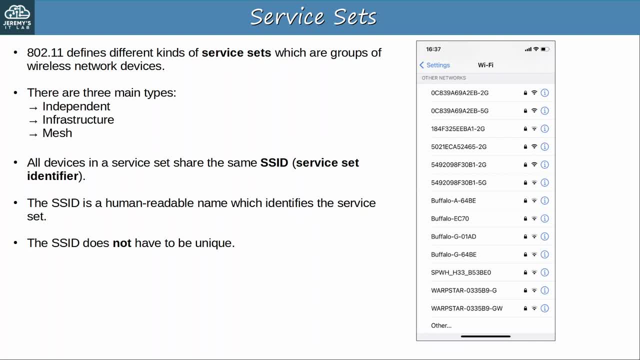 Now, I said, SSIDs are human-readable, meaning they can be given easy-to-read names like Jeremy's Wi-Fi or something like that. In this case, these names aren't exactly the most easily readable. However, I could easily change the SSID of my wireless LAN to something simpler. 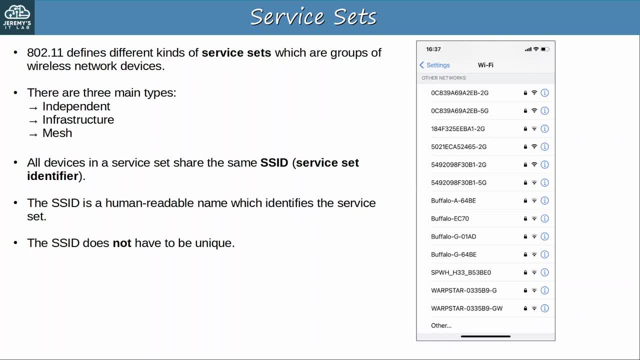 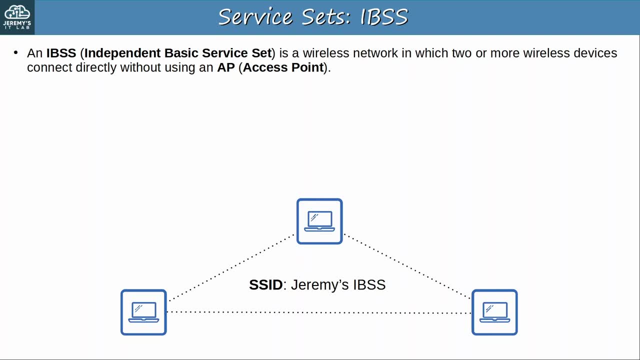 Anyway, let's look at the different types of service sets. First, an IBSS independent basic service set is a wireless network in which two or more wireless devices connect directly without using an AP access point. These are also called ad-hoc networks. 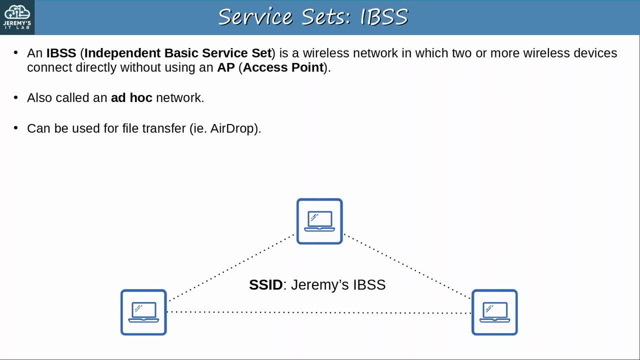 They can be used, for example, for file transfer, such as when using Apple's AirDrop. However, they are not the same. They can also be used for other purposes. They are not scalable beyond a few devices and are typically only used for limited purposes. 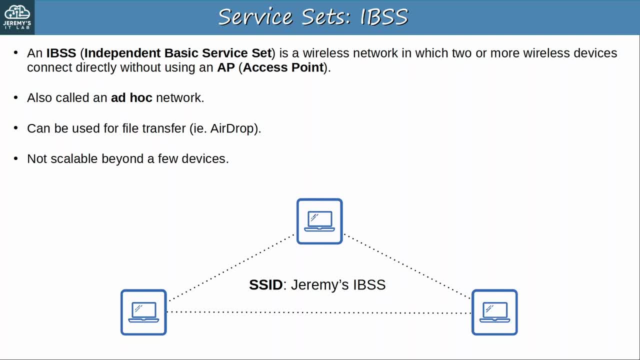 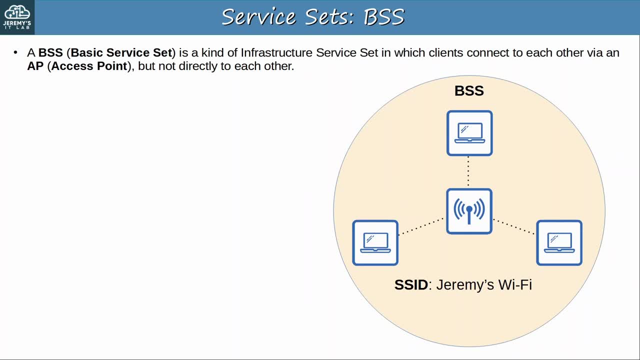 such as quick file transfers like AirDrop. Next, a BSS basic service set is a kind of infrastructure service set in which clients connect to each other via an AP access point but not directly to each other. Remember, I said there are three kinds of service sets. 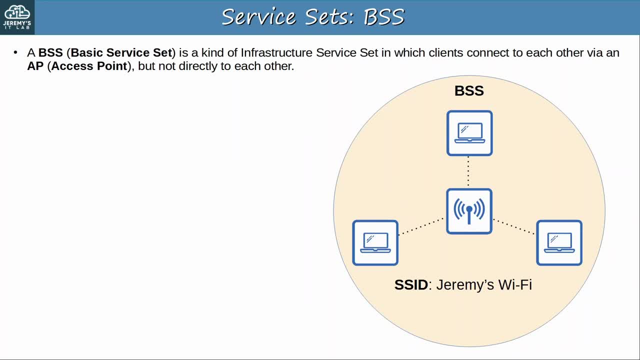 First is independent, which I just showed you, and second is infrastructure. BSS is a kind of infrastructure service. The AP serves as network infrastructure connecting different wireless clients together. A BSS ID- basic service set ID- is used to uniquely identify the AP. 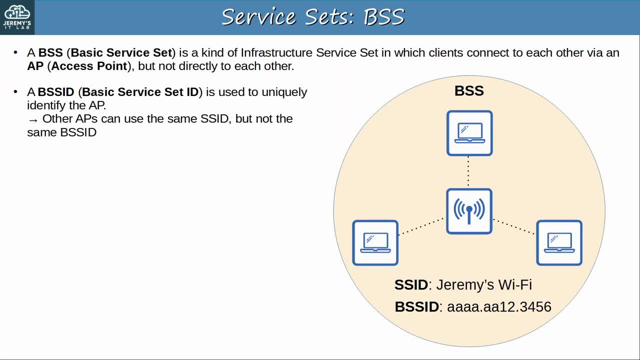 Other APs can use the same SSID, which is Jeremy's WiFi in this case, but not the same BSS ID. The BSS ID is the MAC address of the AP's radio and, as you know, MAC addresses are unique. 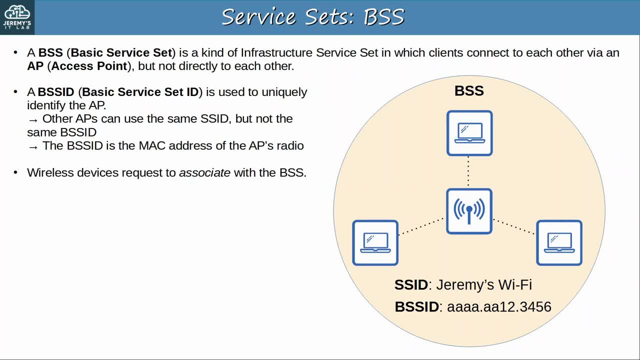 To be part of the BSS wireless devices. request to associate with the BSS. Wireless devices that have associated with the BSS are called clients or stations. Another important term is BSA- basic service area. This is the area around the AP where its signal is usable. 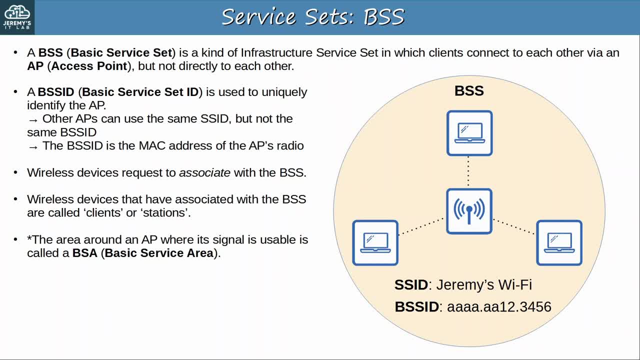 What's different between a BSS and a BSA? Well, a BSS is a group of devices which are wirelessly connected via an AP. BSA just refers to the physical area around the AP where devices will be able to associate with the AP and join its BSS. 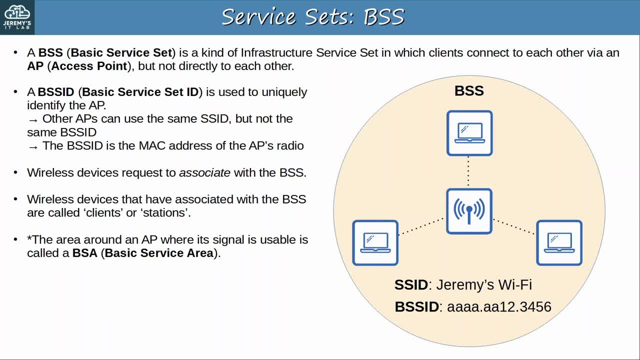 So BSS is a group of devices and BSA is a physical area. And note that clients must communicate via the AP, not directly with each other. The traffic must flow through the AP before going to the other client, even if the other. 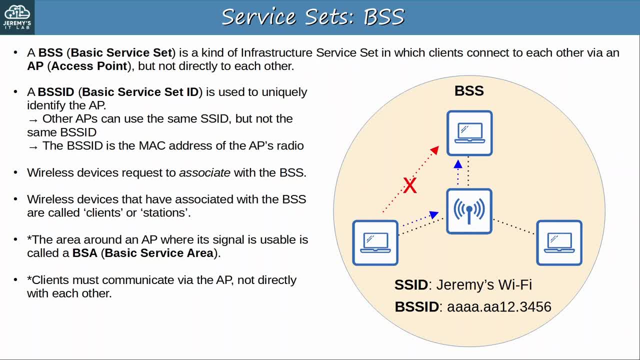 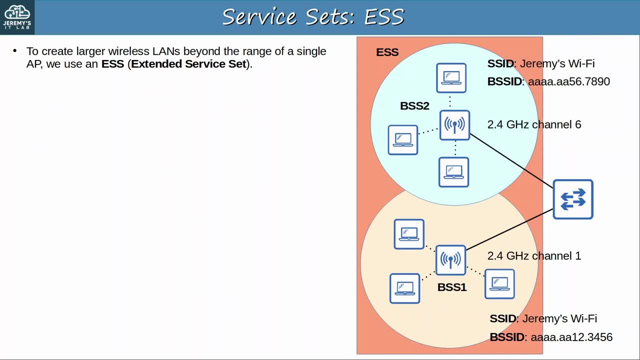 client is in range of the sender's signal. For wireless LANs beyond the range of a single AP, we use an ESS Extended Service Set. This is the second kind of infrastructure service set. Note how there are two BSSs- BSS1 and BSS2, but together they form an ESS. 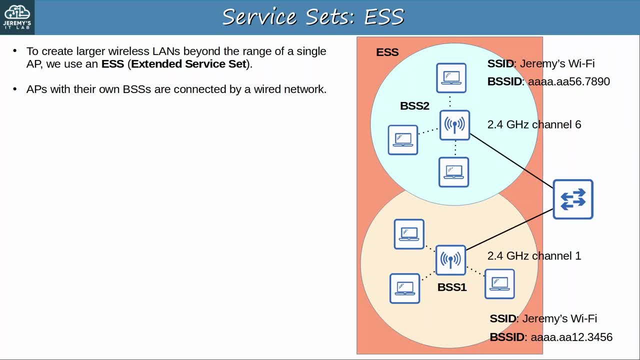 APs with their own BSSs are connected by a wired network. Notice how the APs for BSS1 and BSS2 are connected by a switch. Each BSS uses the same SSID- Jeremy's Wi-Fi in this case. 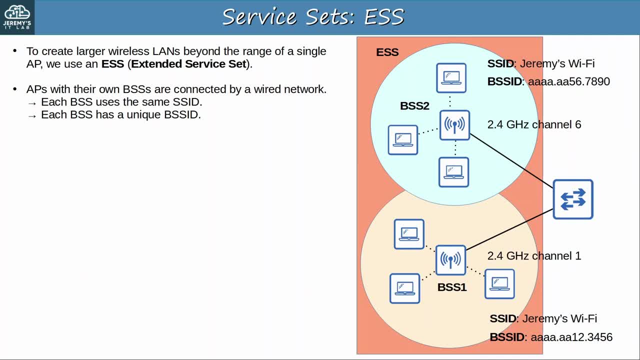 However, each BSS has a unique BSS ID. notice how they are different in the diagram. Also, each BSS uses a different channel to avoid interference. Notice that BSS1 is using 2.4GHz channel 1, and BSS2 is using channel 6.. 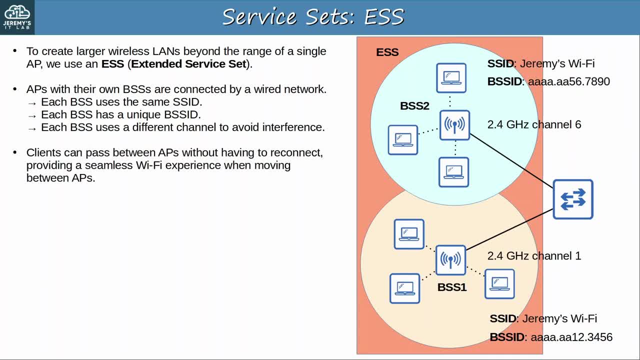 Clients can pass between APs without having to reconnect, providing a seamless Wi-Fi experience when moving between APs. This is called roaming. when you move between two APs in an extended service set, Note that there should be some overlap in the BSAs- about 10-15%- or else the connectivity. 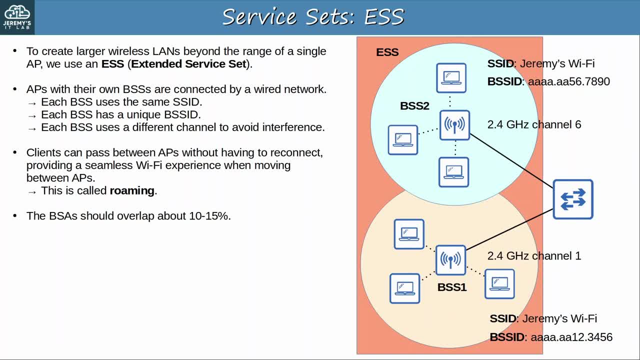 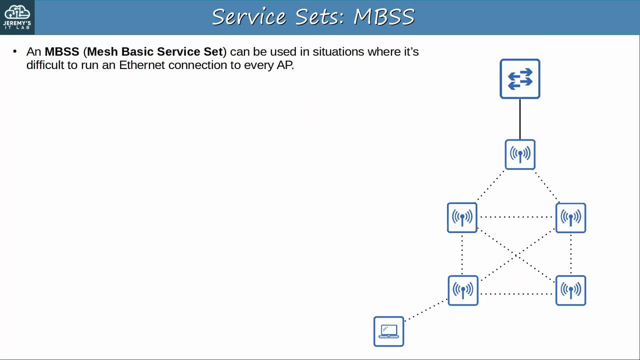 can be lost when moving between APs. The final kind of service set we'll look at is an MBSS Mesh Basic Service Set. An MBSS can be used in situations where it's difficult to run an Ethernet connection to every AP. The MESH APs use two radios. 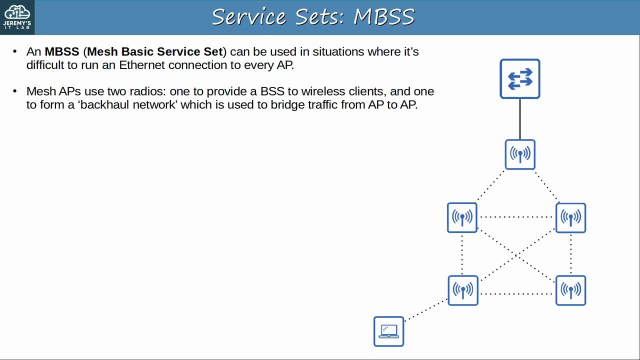 One to provide a BSS to wireless clients so they can connect to the network, and one radio to form the MESH network between the APs, to form a backhaul network which bridges traffic from AP to AP. For example, if this PC wants to send traffic to the Internet, it sends traffic to its nearest. 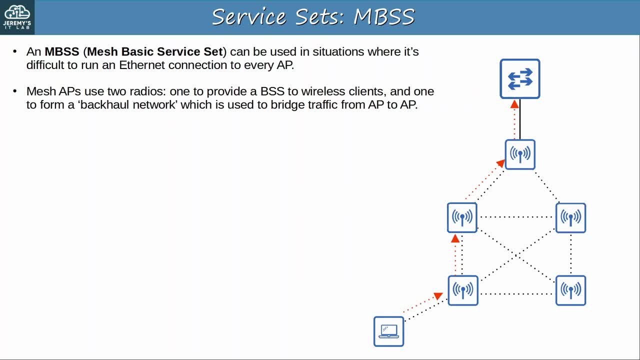 AP, which then bridges the traffic from AP to AP over the backhaul network back to the switch. At least one switch is connected to the wired network and it's called the RAP- Root and Root Access Point. This is the RAP in this network. 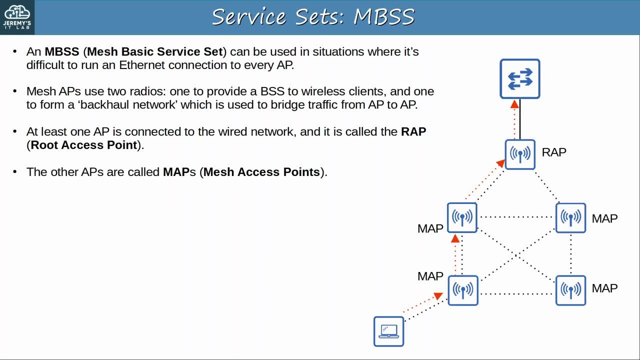 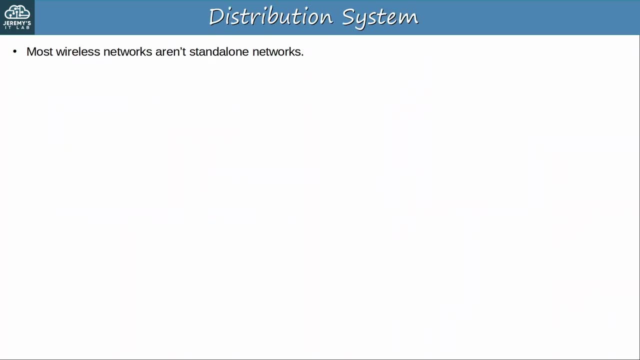 The other APs are called MAPs, Mesh Access Points. A protocol is used to determine the best path that traffic should take through the MESH, similar to how dynamic routing protocols are used to determine the best path to a destination. Now most wireless networks aren't standalone networks. 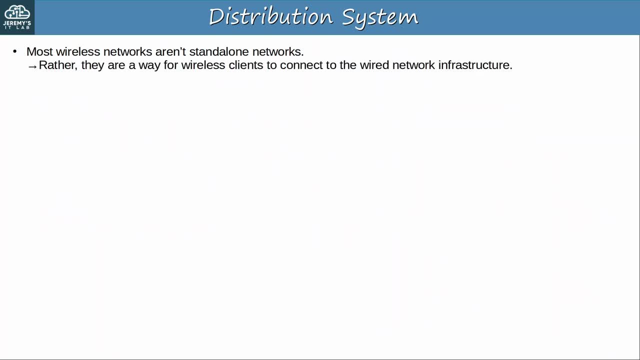 Rather, they are a way for wireless clients to connect to the wired network infrastructure, and the AP serves to translate the network In 802.11, the upstream wired network is called the DS Distribution System. Each wireless BSS or ESS is mapped to a VLAN in the wired network. 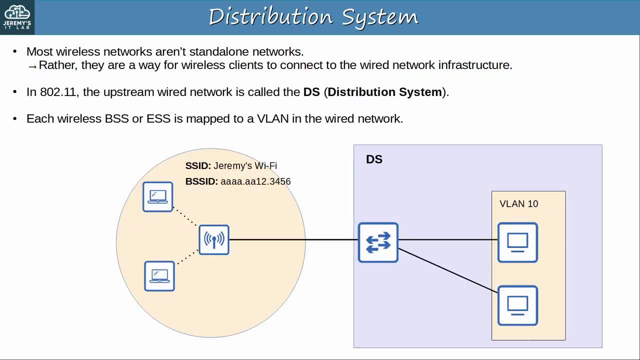 Here's an example. The SSID JEREMYSWIFI is translated to VLAN10. on the wired network, which is the distribution system, The wired hosts in VLAN10 will be able to communicate with the wireless hosts in JEREMYSWIFI. 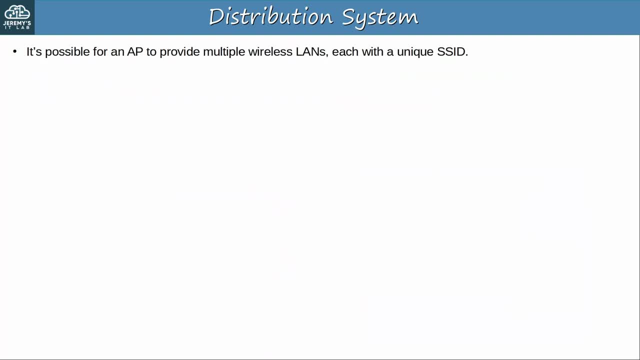 The wireless hosts will be able to communicate with the wireless hosts in JEREMYSWIFI, And it's possible for an AP to provide multiple wireless LANs, each with a unique SSID. This is the same as how a switch can divide a single physical wired network into multiple. 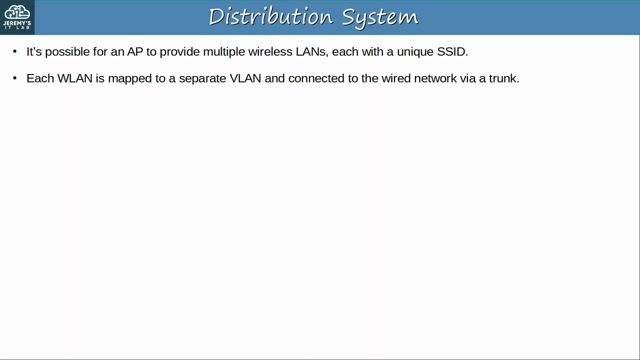 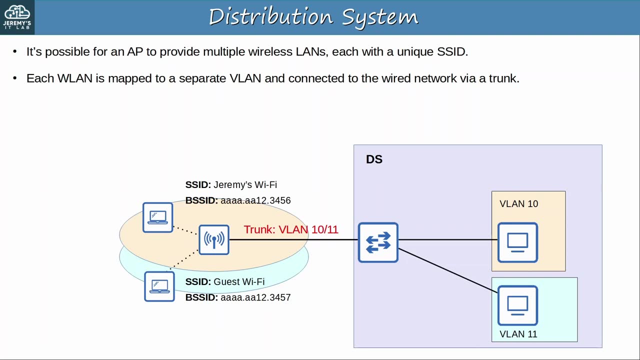 VLANs. Each wireless LAN is mapped to a separate VLAN and connected to the network via a trunk. Here's an example: There are two wireless LANs with their own SSIDs, JEREMYSWIFI and GUESTWIFI, Although, as I said before, SSIDs don't have to be unique. 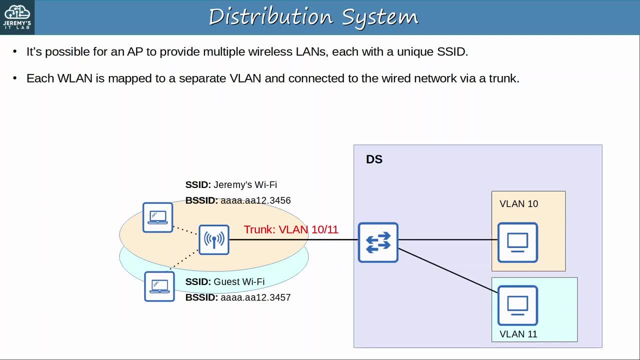 They can be connected to the network via a trunk. Here's an example, But usually they are: JEREMYSWIFI is mapped to VLAN10, and GUESTWIFI is mapped to VLAN11, and the AP is connected to the switch via a trunk which allows both VLAN10 and 11.. 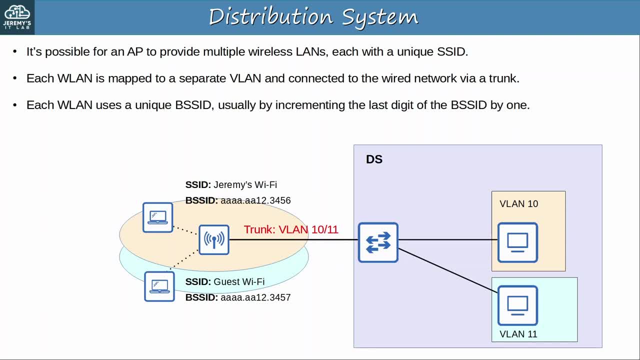 Also notice that each wireless LAN uses a unique BSSID, usually by incrementing the last digit of the BSSID by 1.. So the BSSID of JEREMYSWIFI ends with 3456, and the BSSID of GUESTWIFI ends with 3456.. 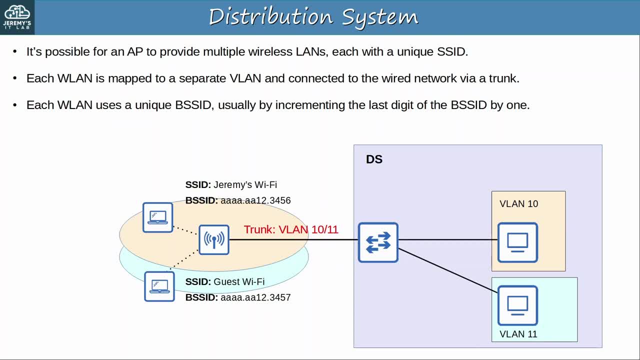 So the BSSID of JEREMYSWIFI ends with 3456, and the BSSID of GUESTWIFI ends with 3456.. The final thing we'll cover is a few more modes that APs can operate in. 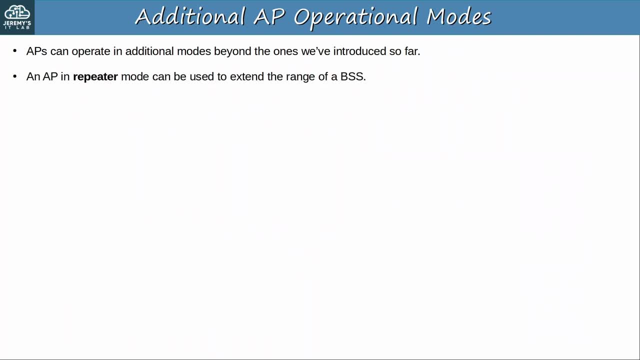 First, an AP in REPEATER mode can be used to extend the range of a BSS. Here's an example: The repeater will simply retransmit any signal it receives from the AP, which will extend the range of the APs- BSS. 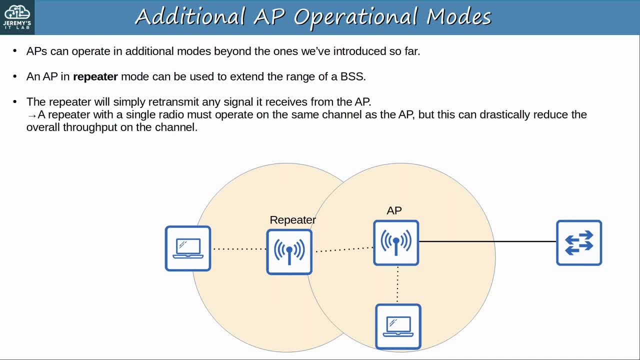 A repeater with a single radio must operate on the same channel as the AP, but this can drastically reduce the overall throughput on the channel channel, since the repeater will be repeating the AP signals back to it using the same channel, keeping the channel busy. 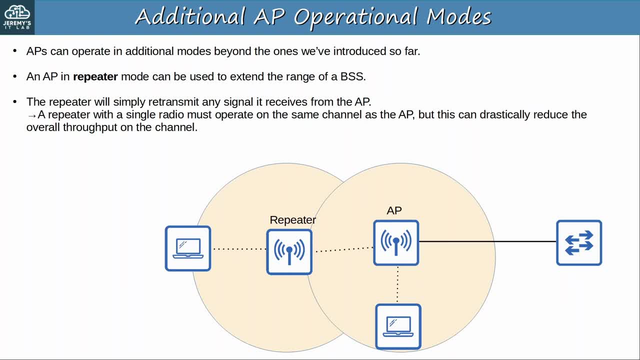 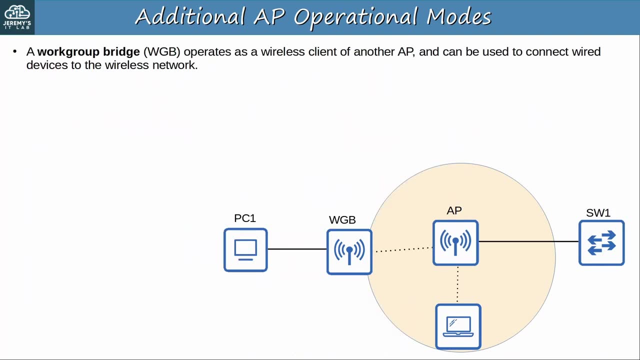 This cuts the effective throughput of the channel by 50%. A repeater with two radios fixes this weakness because it can receive on one channel and then retransmit on another channel. So that's how a wireless repeater works. Next, an AP operating as a workgroup bridge operates as a wireless client of another AP. 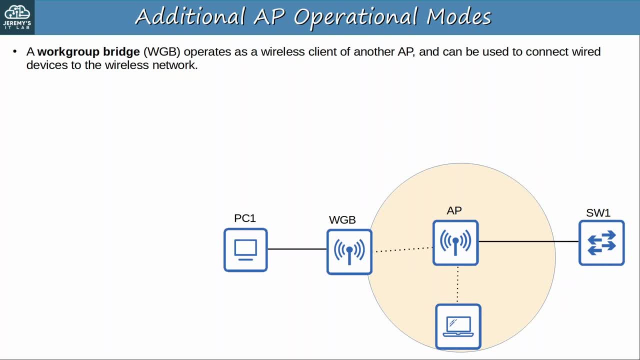 and can be used to connect wired devices to the wireless network. In the example below, PC1 does not have wireless capabilities and also does not have access to a wired connection to SW1.. However, PC1 has a wired connection to the workgroup bridge, which has a wireless connection. 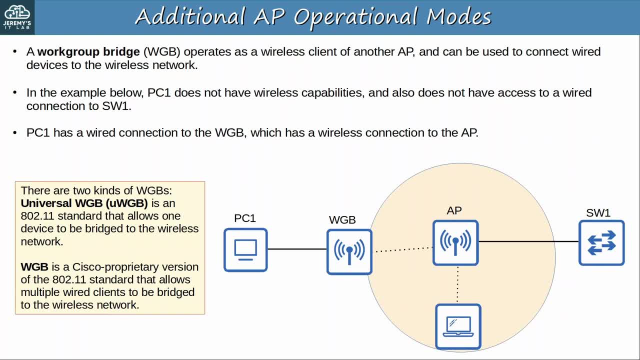 to the AP. Now there are two kinds of WGBs: Universal WGB. UWGB is an 802.11 standard that allows one device to be bridged to the wireless network. However, what Cisco simply calls WGB is their proprietary version, which allows multiple. 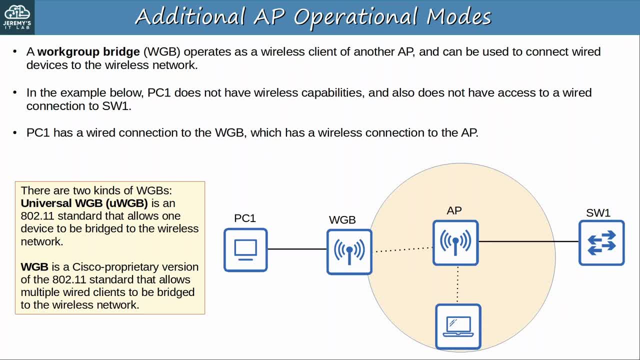 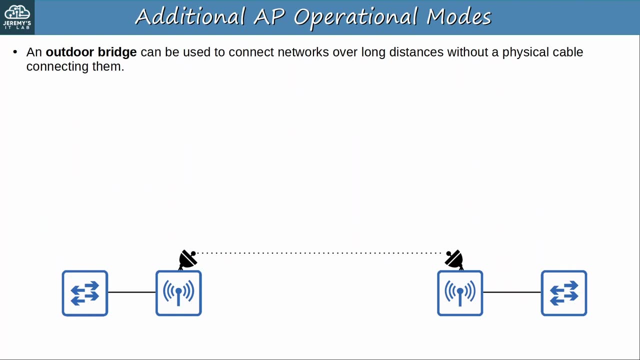 wired clients to be bridged to the wireless network. To summarize, this is a solution which allows clients that don't support wireless connections to connect to the wireless network via an AP operating as a workgroup bridge. The final mode I'm going to introduce is outdoor bridge. 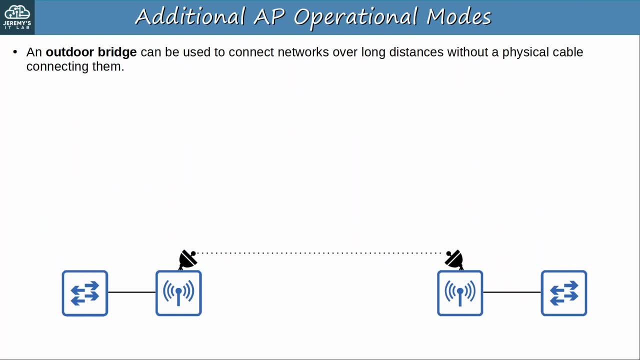 An outdoor bridge can be used to connect networks over long distances without a physical cable connecting them. The APs will use specialized antennas that focus most of the signal power in one direction, which allows the wireless connection to be made over longer distances than normally possible. 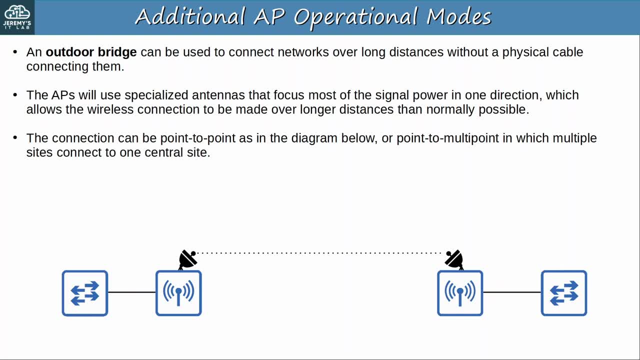 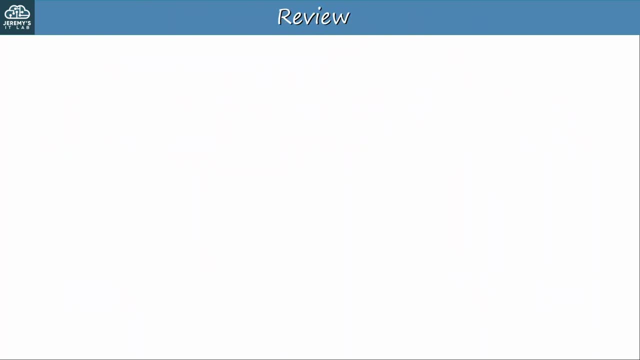 The connection can be point-to-point, as in the diagram, just two sites being connected, Or it can be point-to-multipoint, in which multiple sites all connect to one central site, forming a hub-and-spoke topology. Okay, since we covered so many different topics in this video, let me summarize all of them. 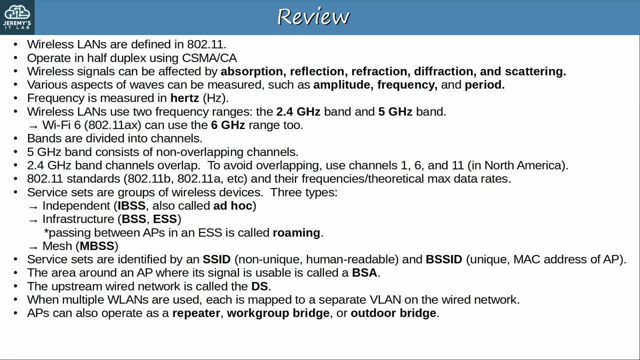 with a lovely wall-to-wall. Here it is Now. although this summarizes the topics in this video, make sure you know the details of each topic that we covered. If you didn't take notes, I recommend going back in the video to take your own notes. 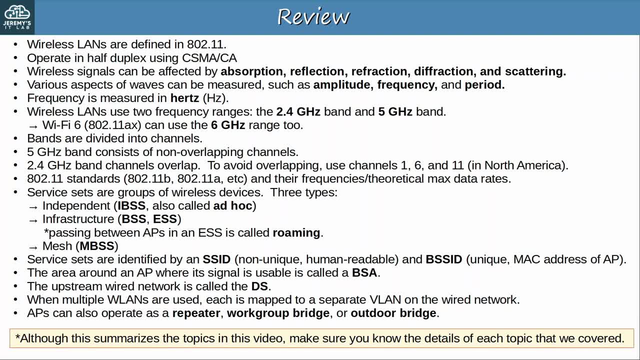 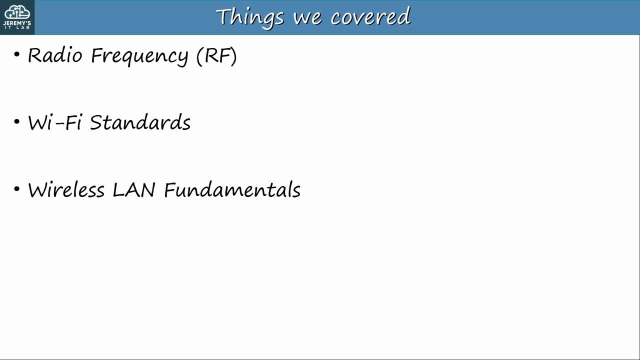 and also using the flashcards to memorize some of the details. Okay, in this video we covered the basics of wireless networks, specifically wireless LANs, including radio frequency Wi-Fi standards, and wireless LAN fundamentals such as service sets. There is still a lot more to cover about wireless networks, including wireless network. 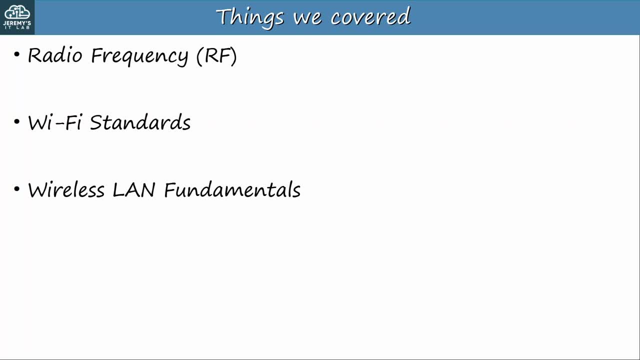 architectures, wireless network security and wireless network configuration. Those topics will be in the next few videos. As always, watch until the end of the quiz for a bonus practice question from Boson Software's ExSim for CCNA. the best practice exams for the CCNA. 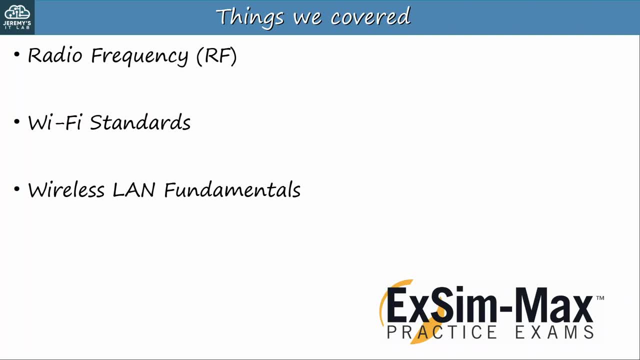 Okay, let's go to quiz question 1.. When using the 2.4GHz band, which channels should be connected to each other? Let's start with the 2.4GHz band. Let's start with the 2.4GHz band. 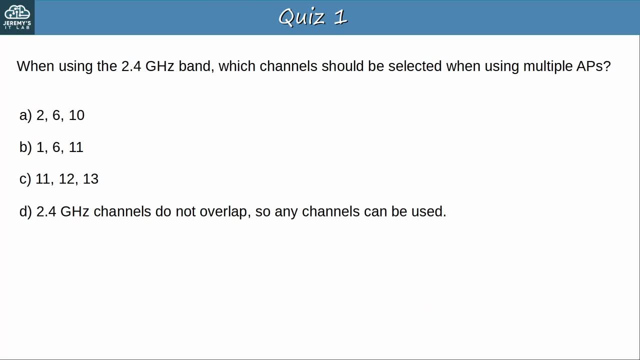 What network should be selected when using multiple APs? Pause the video now to select the best answer. Okay, the answer is B, 1,, 6, and 11.. As this diagram shows, channels 1,, 6, and 11 do not overlap, so even if APs are near. 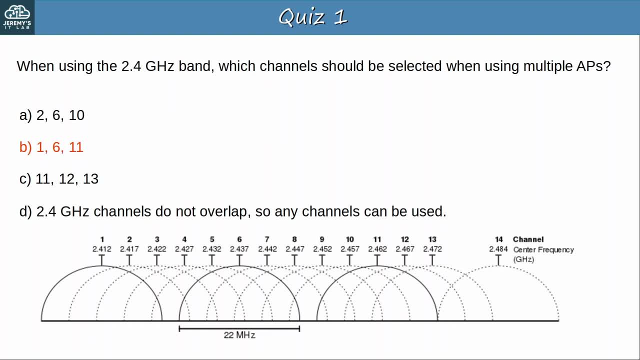 each other. interference can be avoided. Okay, let's go to question 2.. What network should be connected to each other? Let's go to question 2.. What network should be connected to each other? Let's go to question 2.. 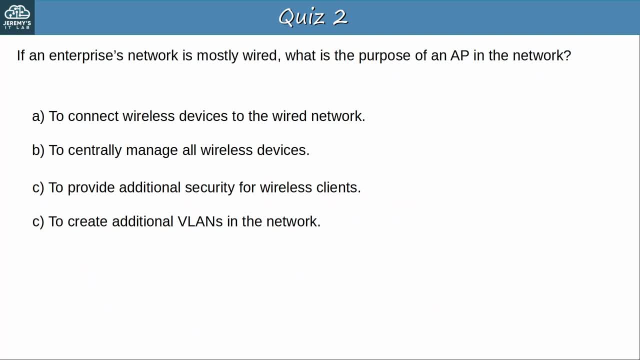 What network should be connected to each other? what is the purpose of an AP in the network? Pause the video now to select the best answer. Okay, the answer is to connect wireless devices to the wired network. In 802.11,, the wired network is called the DS distribution system and the AP's main role. 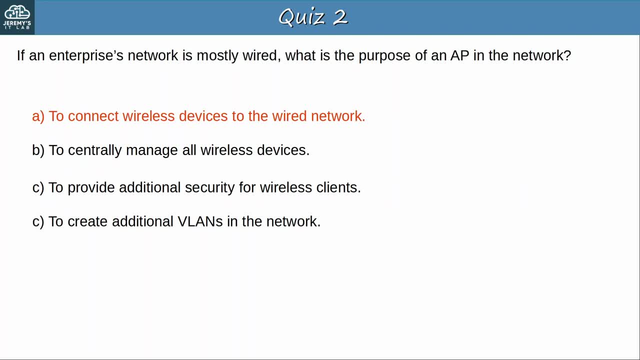 is to connect wireless devices to the wired network. Okay, let's go to question 3.. Which of the following bands are commonly used by wireless LANs? Select two. Pause the video now to select the best answers. Okay, the answers are A- 2.4 GHz and D- 5 GHz. These bands are divided into channels which are: 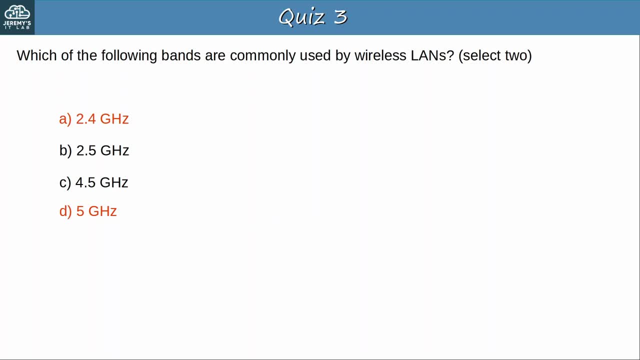 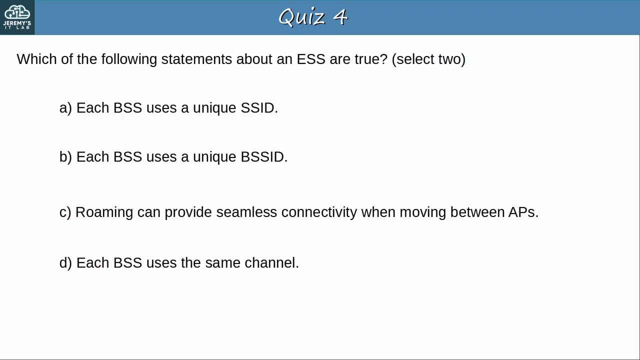 used by wireless devices to send and receive wireless signals. Okay, let's go to question 4.. Which of the following bands are commonly used by wireless LANs? The following statements about an ESS are true: Select two. Pause the video now to select the best answers. 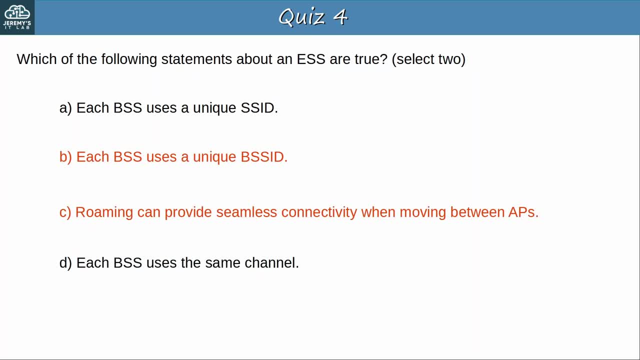 Okay, the answers are: B- each BSS uses a unique BSS ID, and C- roaming can provide seamless connectivity when moving between APs. A is not correct because each BSS in an ESS should use the same SSID, and. D is not correct because adjacent APs should use. 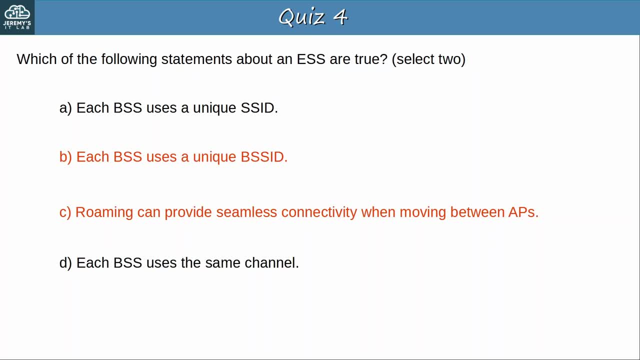 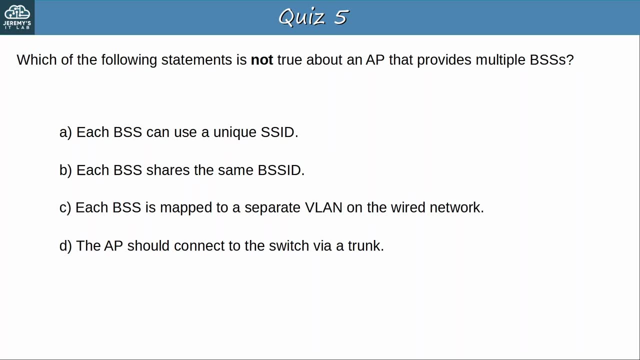 the same SSID. Both are possible, but B is not correct, because sometimes the APs are connected to one of the same overlapping channels to avoid interference. Okay, let's go to question 5.. Which of the following statements is not true about an AP that provides multiple BSSes? 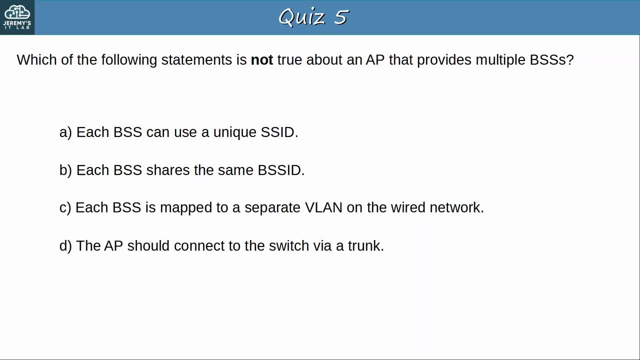 Pause the video now to select the best answer. Okay, the answer is B. Each BSS shares the same BSS ID- unique BSS IDs. With that said, however, it is best practice to also use a unique SSID for each. 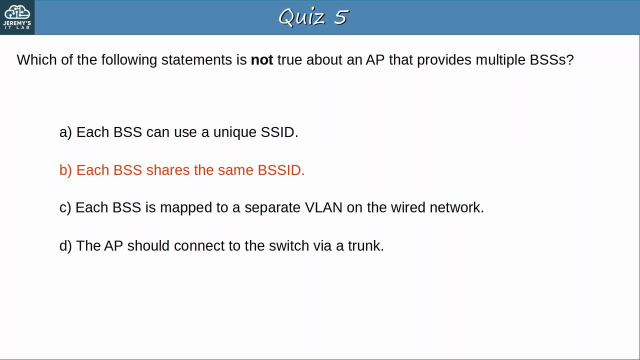 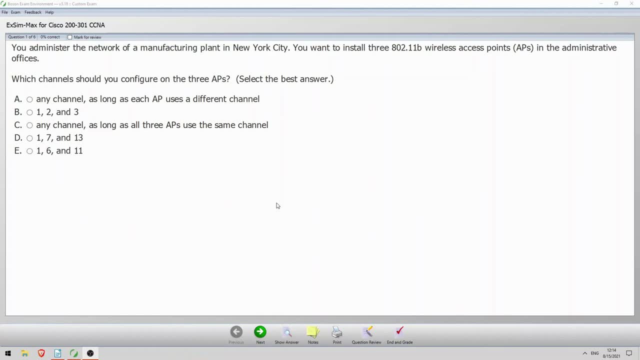 BSS. Okay, that's all for the quiz. Now let's try a bonus practice question in Boson Software's ExSim for CCNA. Okay, here's today's Boson ExSim practice question. You administer the network of a manufacturing plant in New York City. You want to install three 802.11b wireless access points. 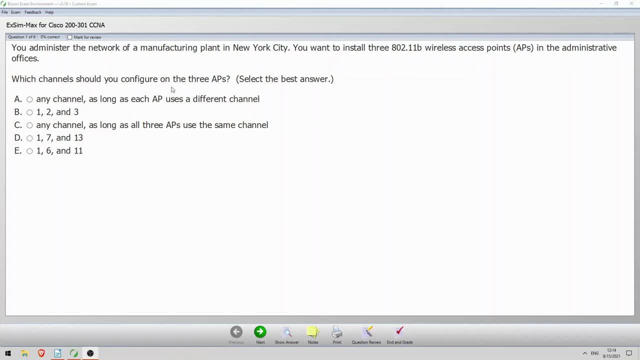 in the administrative offices. Which channels should you configure on the three APs? Select the best answer. Okay, pause the video now. check out the options and select the best answer. Okay, let's check. So this is actually very similar to one of the questions I just asked. 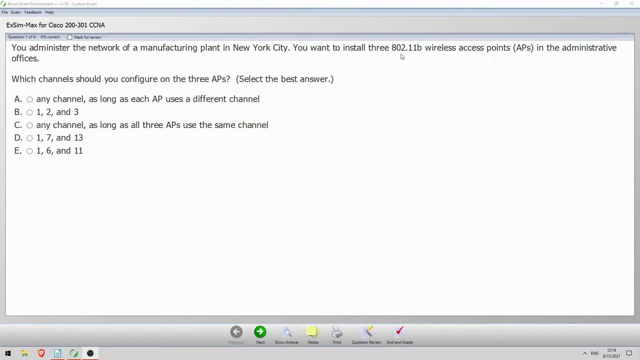 in my quiz. So the problem is: you have to know what frequency, what band 802.11b uses. If it uses the 5 GHz band, the BSS is the best answer If it uses the 5 GHz band. 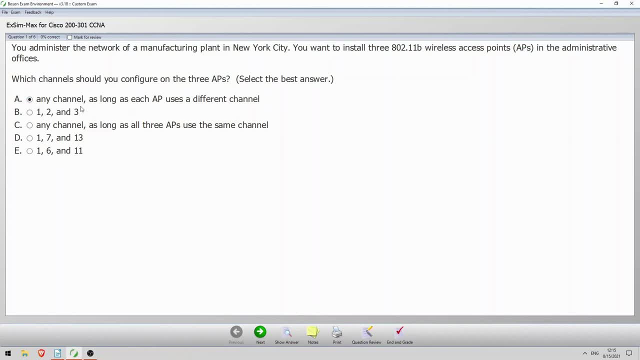 the BSS is the best answer If it uses the 5 GHz band. the BSS is the best answer If it uses the 5 GHz band. the answer should be A, any channel, as long as each AP uses a different channel. That's because the 5 GHz band is divided into channels that don't overlap, so it doesn't really matter which channels you use, as long as they don't overlap. But if 802.11b uses the 2.4 GHz band, then the answer. 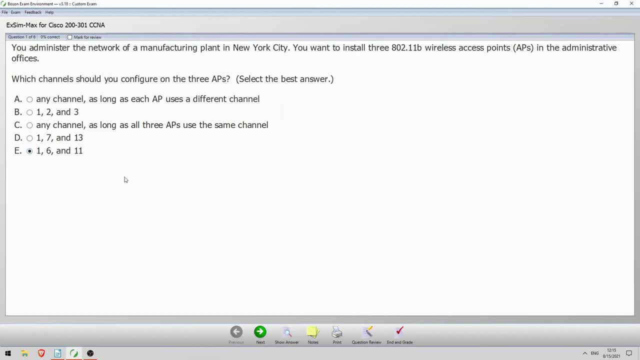 should be 1,, 6, and 11, because the 2.4 GHz band is divided into channels that do overlap, So you don't want any of the channels to overlap. So if 802.11b uses the 2.4 GHz band, then the 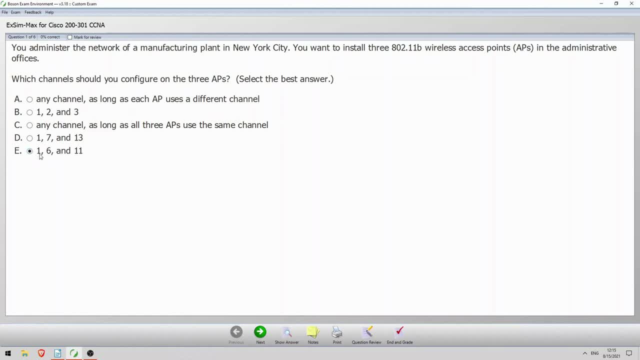 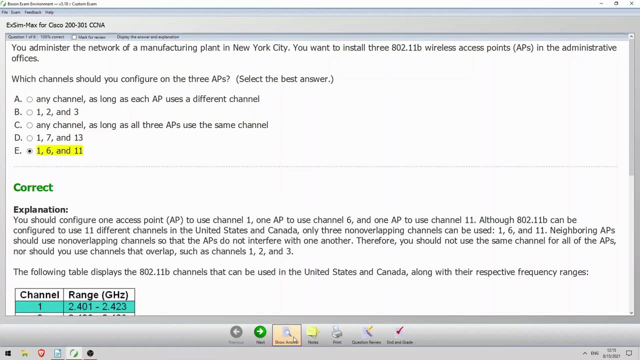 you don't want any of the channels to overlap. So you don't want any of the channels to overlap, So you should use channels 1, 6, and 11, because those channels don't overlap. Okay, so let's check the answer. Okay, the answer is E. so that's because 802.11b uses the 2.4 GHz band. 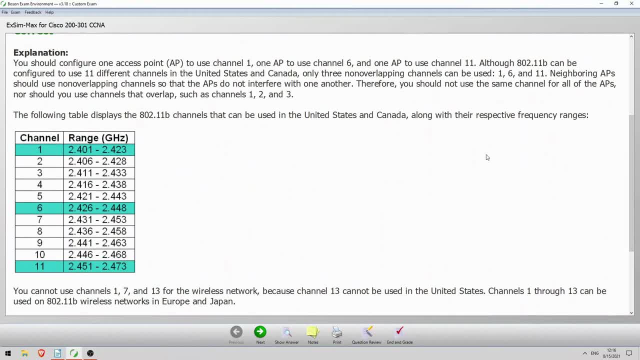 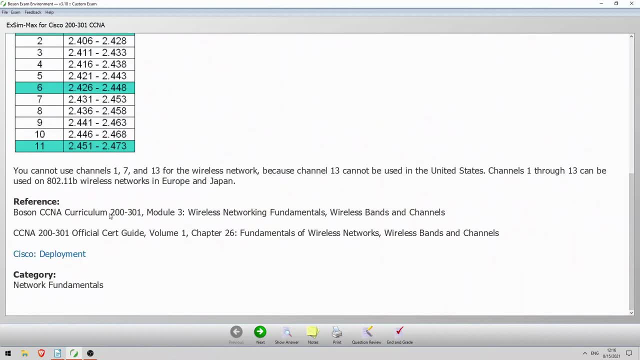 Okay, so here is Boson's explanation. I recommend pausing the video now to read it. Okay, let's check the references. so they have references to Boson's explanation. so they have references to Boson's explanation. so they have references to Boson's own CCNA curriculum. 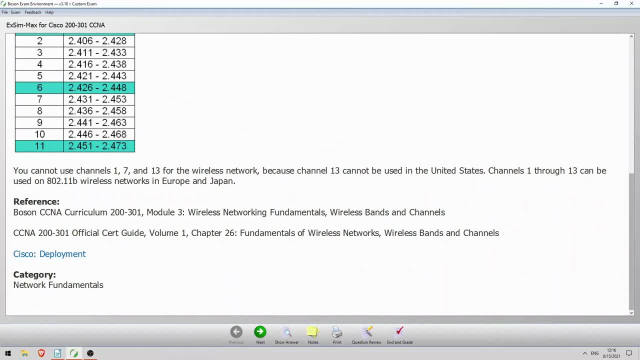 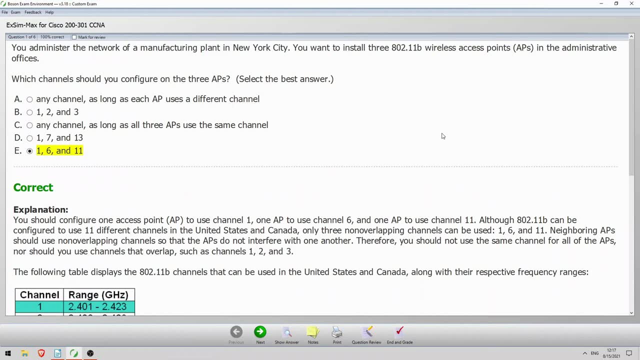 the official cert guide and a Cisco wireless deployment guide. Okay, so that was a quick look at Boson Software's ExSim for CCNA. As I've said before, these are by far the best practice exams for the CCNA If you want to get Boson ExSim. 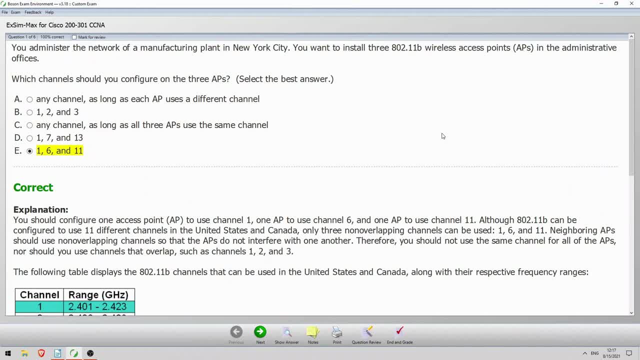 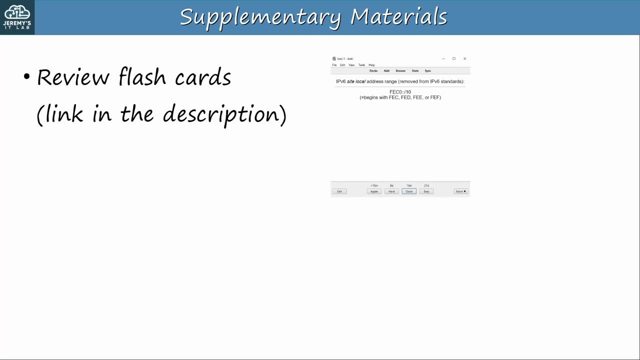 please follow the link in the video description. There are supplementary materials for this video. There is a flashcard deck to use with the software Anki. There won't be a lab for this video but I'll put a link to it in the description. 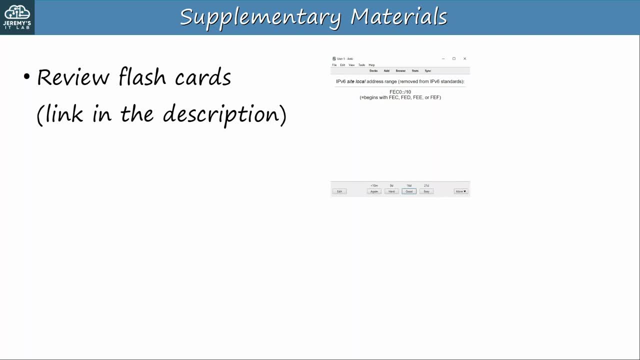 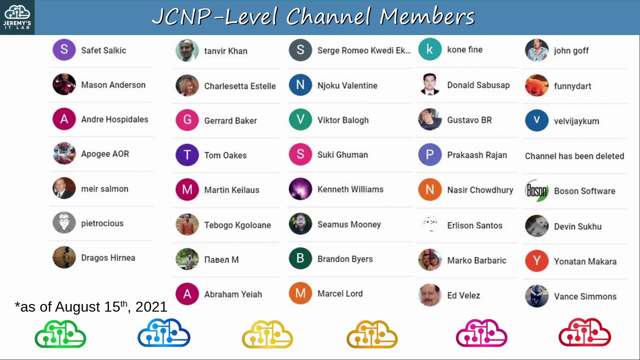 We covered some of the fundamentals of wireless networking, but no configurations yet. That will be covered in a future video. Before finishing today's video, I want to thank my JCNP-level channel members To join. please click the join button under the.